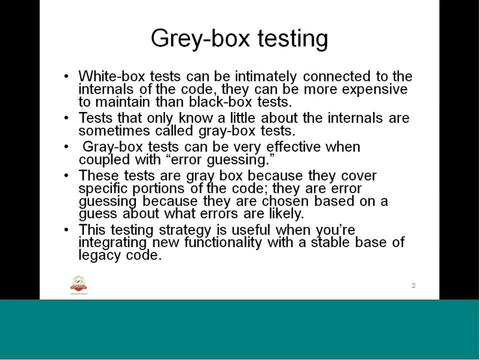 tester has a knowledge about internal details of the system as well as the system knowledge. with the help of that and he will do the testing. This is actually very effective when it is coupled with error guessing where, with the help of the system knowledge, he will guess. 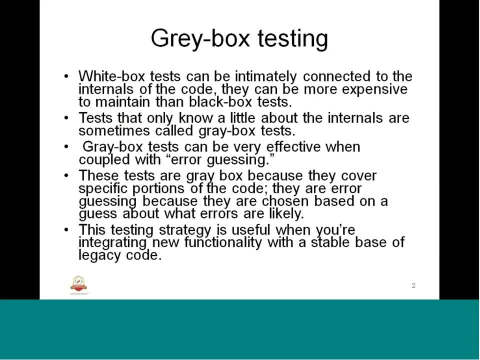 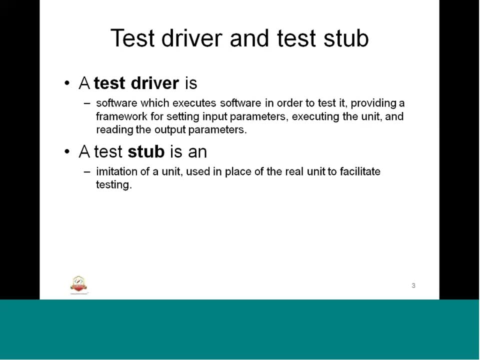 what sort of errors could come. This is particularly useful when we have a stable system, knowledge, The system working with the legacy code and there are certain changes or new functionality has been added to the embedded system. Also, we studied about test driver and test hub, which is a very important part of the embedded software. testing Test driver is: 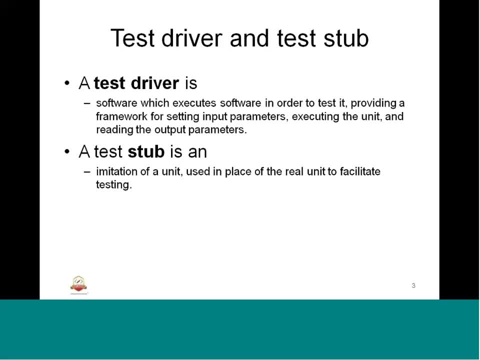 software which executes software in order to test it, providing a framework for setting input parameters, executing the unit and reading the output parameters. So basically, test driver will invoke the test which we want to test it. There is also a software piece with whatever the values that we want to provide as inputs. 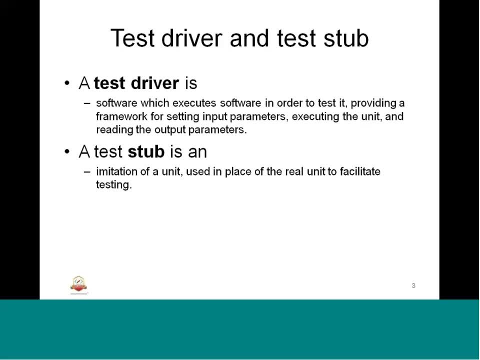 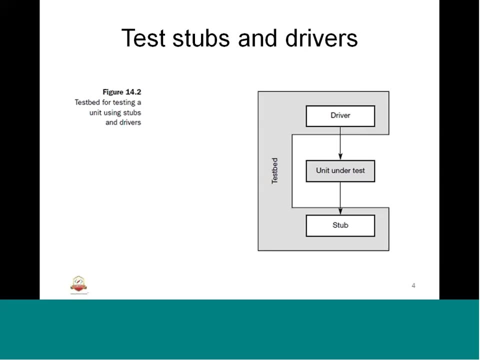 and expect the outputs. Test hub is a replacement of the existing unit, So this is used in place of the real input to facilitate the testing. So this is the framework that is being used for test hub and test driver. This is called a test bench or test bed, basically. So the 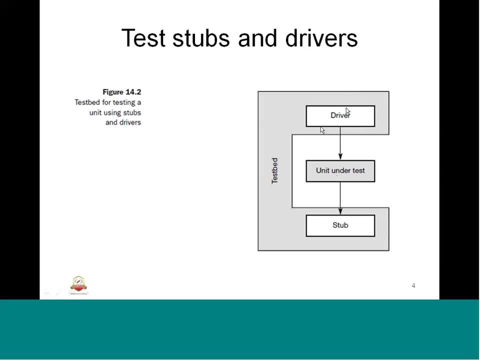 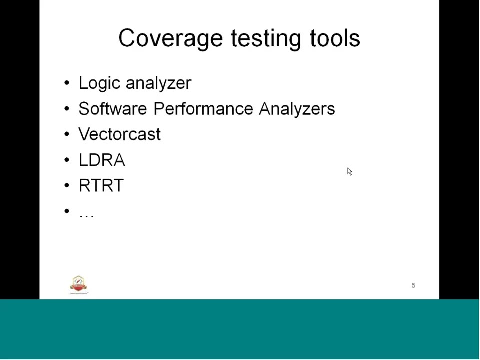 unit is getting used by driver And unit can be replaced with the help of a test hub. So test hub and drivers are part of the test bed and the unit will be subject to the test. Coming to the various aspects of the tools that are used in white box testing, Basically, 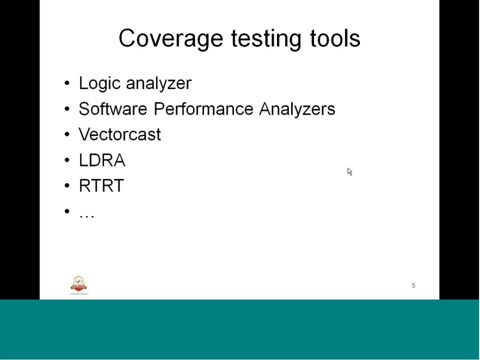 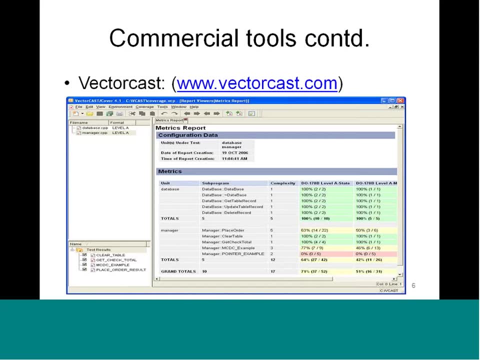 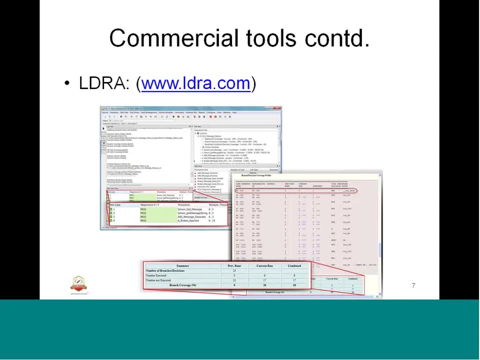 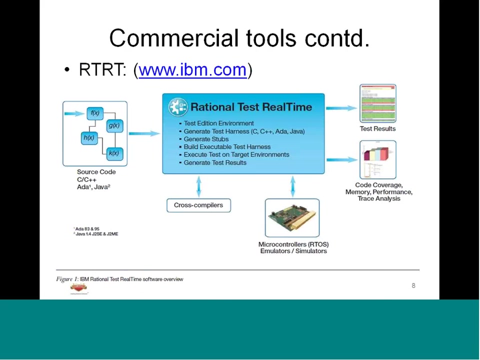 they use for coverage purposes and we have studied about commercial tools such as vector cast for covering, for getting the reports of the coverage, And we also went through 3d array from 3d arraycom and IBM rtmt, which is has facility for doing the test hubs, building the executable from the target and generating the reports. 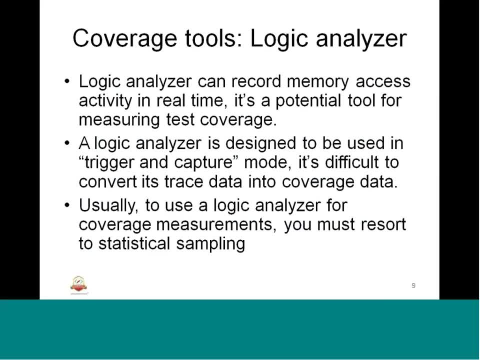 Also we studied about logic and measure, which will help in recording the memory activity in a right way. So we have studied the logic and measure which is used in marking in the changes and the updates that are happening in the ML software. it basically captures: 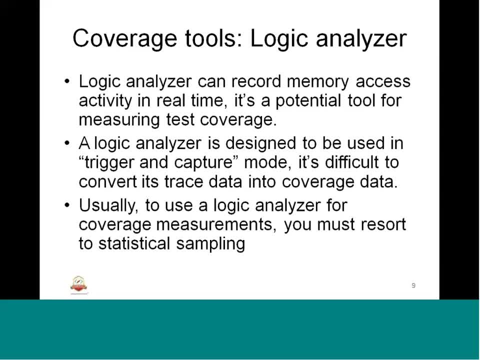 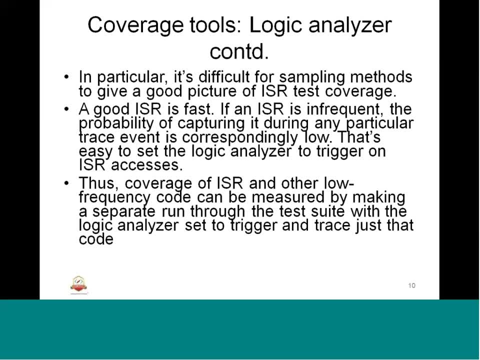 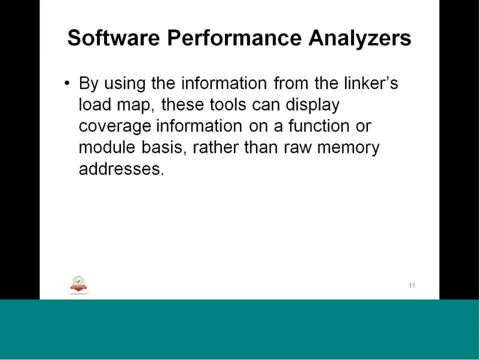 the events that are happening and it is called a trace. it is particularly useful for interrupt based applications, where more inputs are there and frequency of the interrupts are more. Also, we had a study about software performance analyzers. the performance could be from memory. 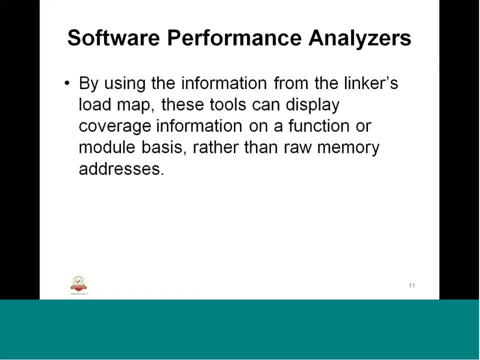 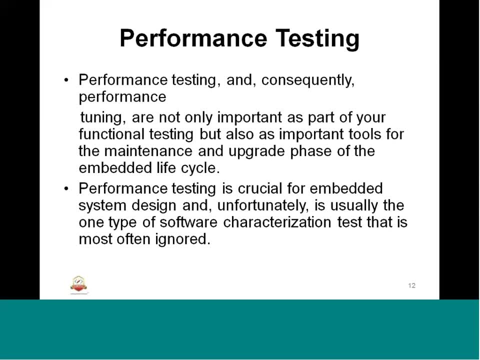 timing and the load speed etc. so performance testing and tuning is very important aspect because that will try the functionality and especially if the software has to be upgradable or memory enable. So the performance testing is very important aspect because that will try the functionality. 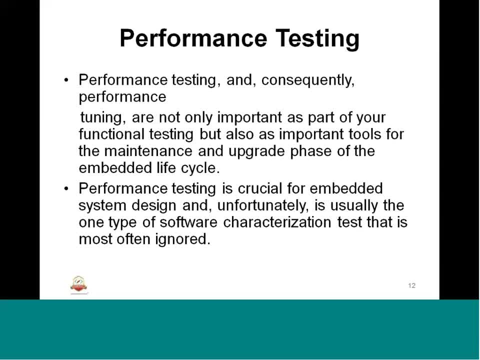 and especially if the software has to be absolutely right, then only we can do the rest of the testing. So these are very important aspect but sometimes in the industry this will be taken as a last priority. but as per me this should be a top most priority for doing the ML software testing. 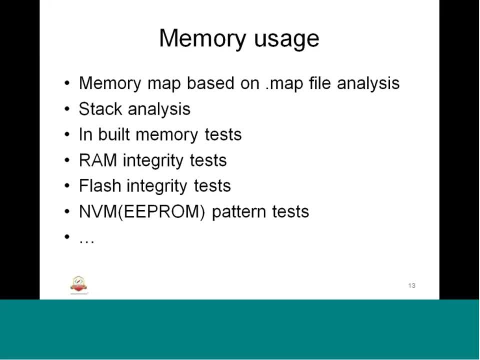 Also, there are various types of memory testing. we do So especially. they look for the memory usage, how the memory is being used in the ML software testing, embedded software system and there is a map file, and the map file will be detailed in terms of how much stack, how much constants are using, what is the size of the RAM, what. 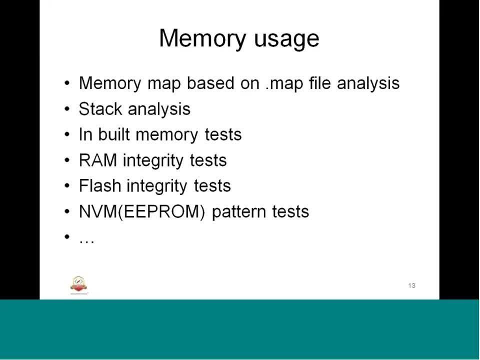 is the size of the flash, etc. And for testing each of these memory parts within the embedded software. basically, the software itself will have a and it will keep on checking in every fixed intervals or cycles of the system life and the reports will be generated or hooked with the external tool. 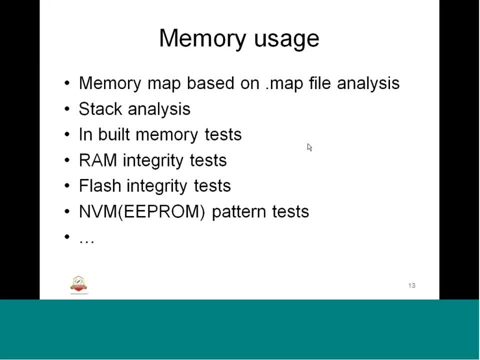 to get the data and that will be analyzed. So basically, the RAM, the memory flash, will be checked with the help of integrity tests. integrity test could be working ones or pattern tests. NVM also will be tested with the help of pattern test or working one test. 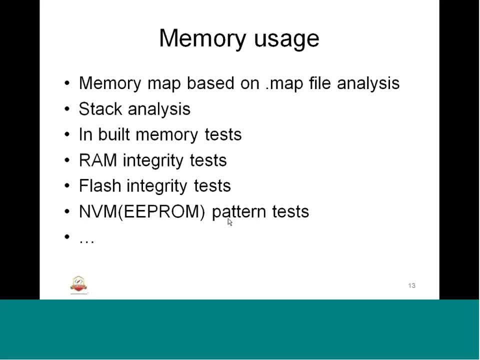 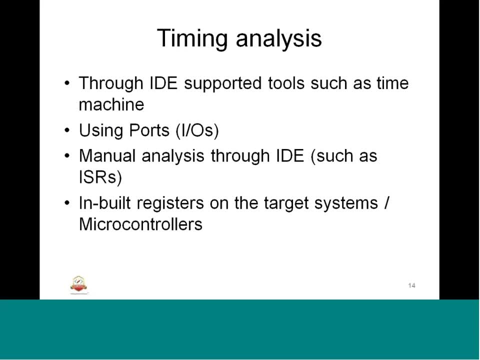 So this is where the E-Scope ROMs are used: for fault, for recording and storage And timing analysis we can do with the help of integrated development environment. with the help of the debuggers, we can analyze the inputs and the various events that are happening. 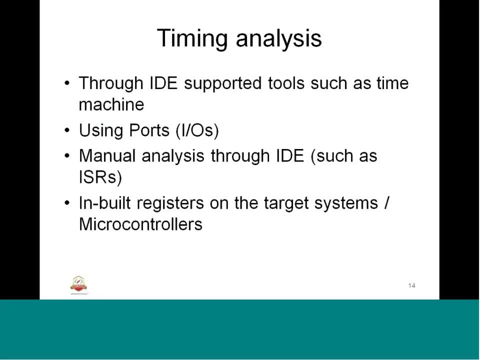 with respect to time and as a black box. so if you want to test it, you may have to use ports, if it is available within the embedded system and those ports can be scoped using the E-Scope. ROMs And E-Scope will be analyzed with respect to the plotted graph of timing. with respect. 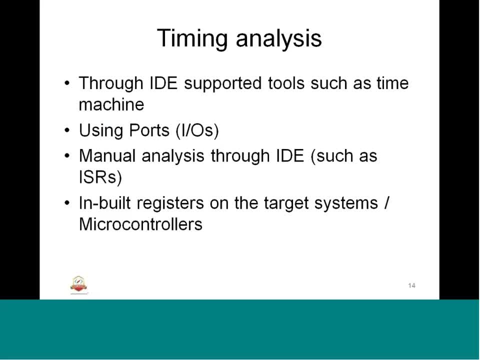 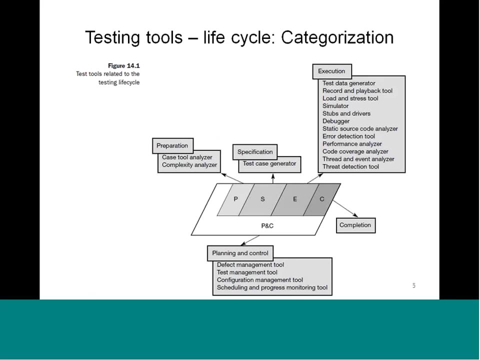 to various events. also, the embedded system has registers with respect to time, such as RTC, watchdog, etc. those will be used as well in terms of analyzing time. Also, we went through the testing tools life cycle, how the life cycle has been used. The life cycle can be used with respect to the tools, so we have a planning and control. 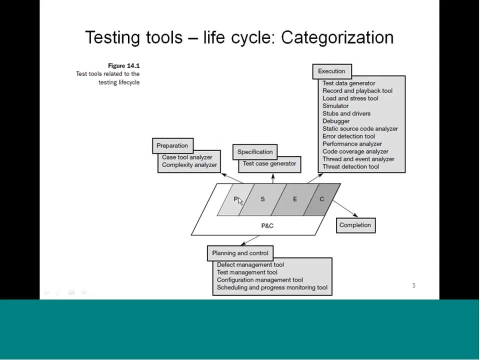 of the entire testing life cycle which has a preparation, specification, as we call it, and completion. So preparation, we have tools such as case tool analyzer, complexity analyzer. for specification, we have test case generation or test case computer which has Perl or Python scripts or Excel sheet programming from the requirement. 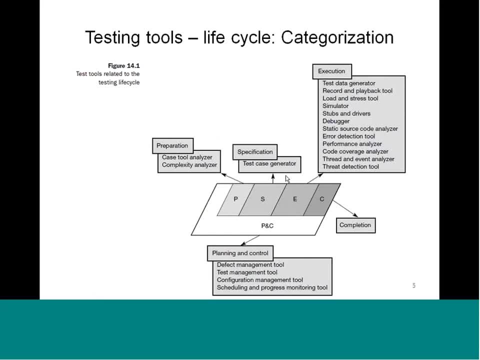 So these are the tools we have. Thank you, Thank you, Thank you very much. And the other thing which we have done, so we have execution in terms of test, data generator, simulators, debuggers, whatever we have studied so far. 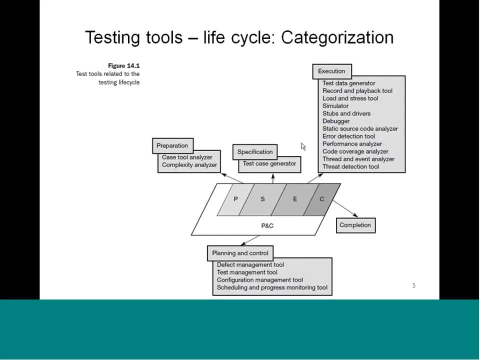 One of them or many of them could be used for execution purpose And we have the completion and reporting mechanism of the executed parts For planning and control. we used management and test, management and traceability, etc. These are the tools, Thank you, etc. with respect to the requirements for testing. 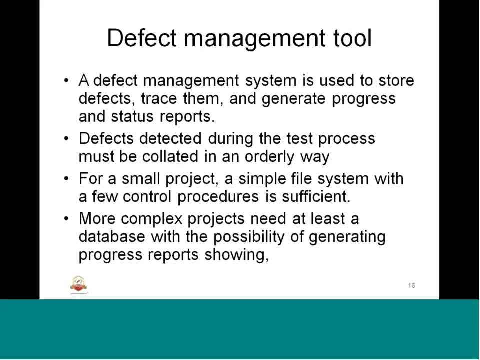 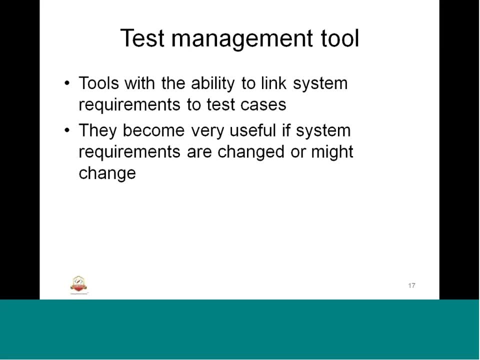 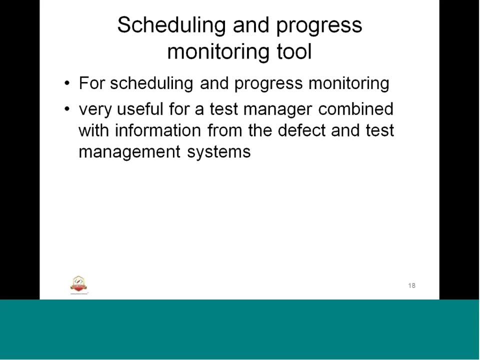 Defect management we have, depending on the size of the project, the type of defect, complexity and all that will be managed with the database and all that. they will be used in order to get the report of the defects, as well as the requirements, accessibility And in terms of scheduling and all that. they use different types of tools such as MPP and 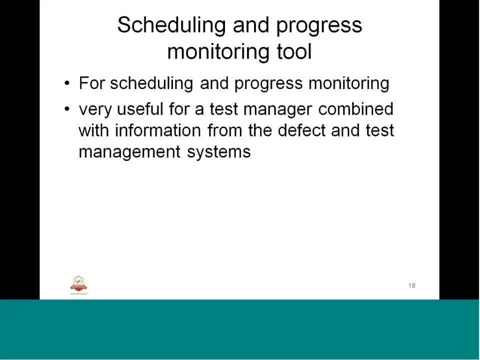 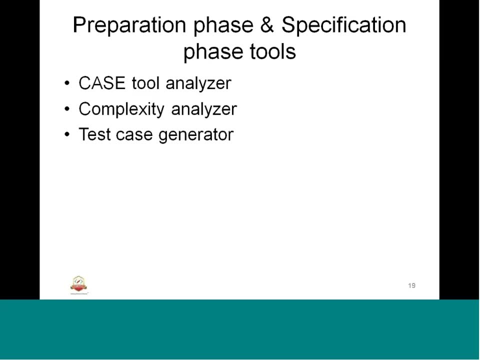 test link, bugzilla, whatever it is, can be used in addition to scheduling. This will help test management and progression of the embedded softwares. testing, Test, case preparation, specification, then, with the help of case tool analyzer, complexity analyzer, In case generators for specification, they use it. 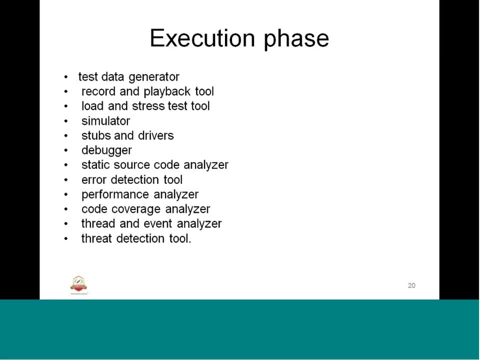 Execution. we have seen stops and driver emulators, emulator debugger, static code analyzers, performance analyzer, timing analyzers, code coverage analyzers are used. These are all basically using white box testing as well as black box testing. Okay, 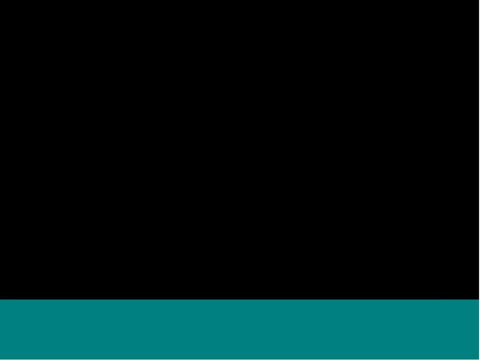 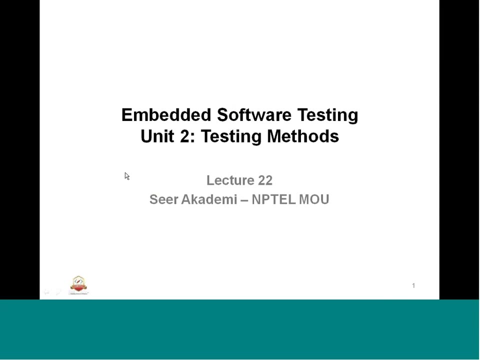 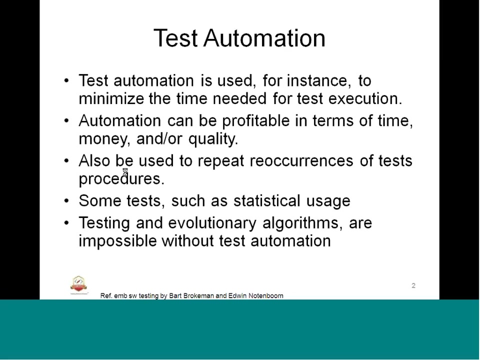 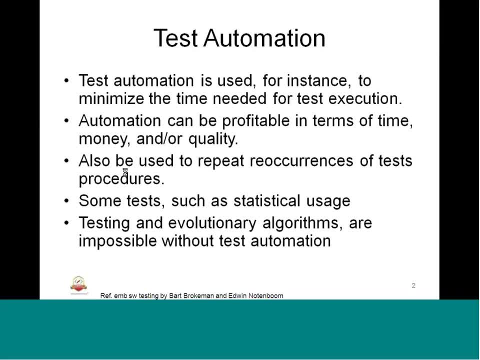 implemented and how they can be executed and in what way we can automate it. So, basically, test automation is a process or test method or whatever. Okay, Okay, Okay, Okay, Okay. So the test automation is used to minimize the time needed for testing. 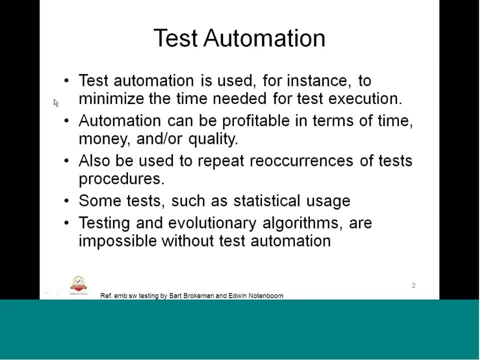 So why we need a test automation is we will keep on doing the embedded software testing again and again, and similar requirements, similar setup of things. So we need to have a common framework. Okay, Okay, Okay, the entire system to test and will feed the values with respect to each test cases and 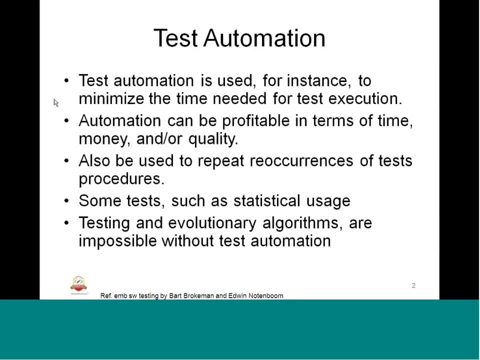 that is why the test framework, along with execution test automation, is useful. So automation is very profitable in terms of time, money and quality, but it needs a initial investment of time. one time once it is done, the framework is available, it is very easier to maintain as well as run the test automatically. 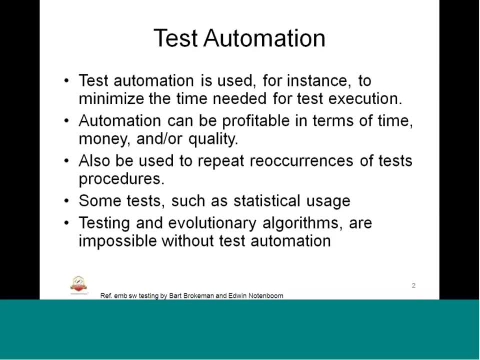 So very less human intervention is required in terms of testing and also it can be used to repeat reoccurrences of test procedures. that means so multiple tests of similar procedures. we do not need to do it manually, we can do a batch processing, batch automation it is. 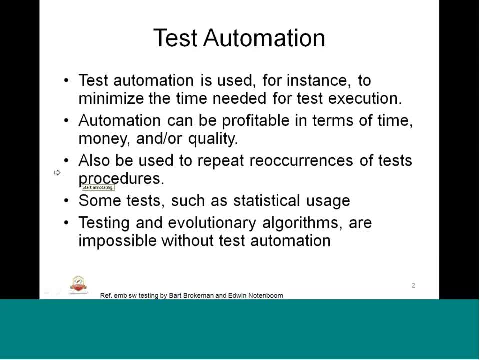 very simple. So test automation will help in doing these things where multiple procedures are to be executed in a batch, and some tests, such as statistical or usage, also can be done with the help of test automation. Testing and evolutionary algorithm are impossible without test automation. that means there are 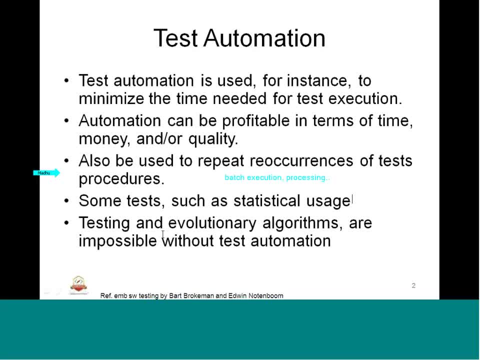 certain things Which are of repetitive nature, so algorithms which keep changing. we have a set of data and there are fixes and we may have to do regression, so we cannot afford to have a manual effort again and again spent on that. so in that way it is very useful to have test automation. 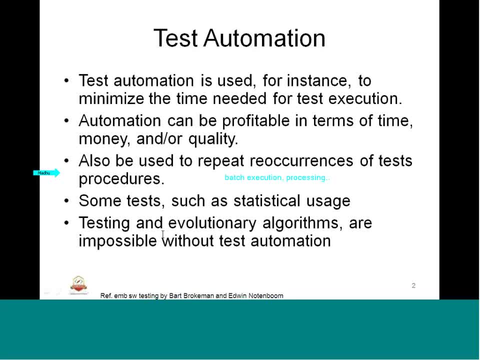 So basically, in principle, the execution of almost every test can be automated, depending on type of test In fact. if so, only a small part of the tests are automated in depending on the project again, but the automation will be done most of the requirements where similar functionality. 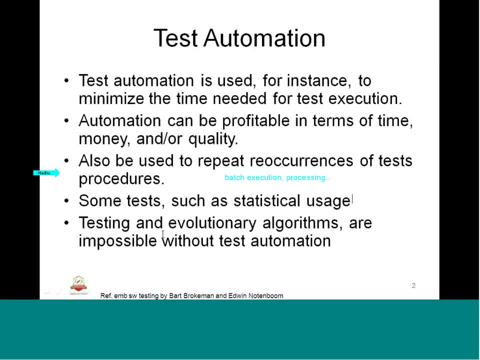 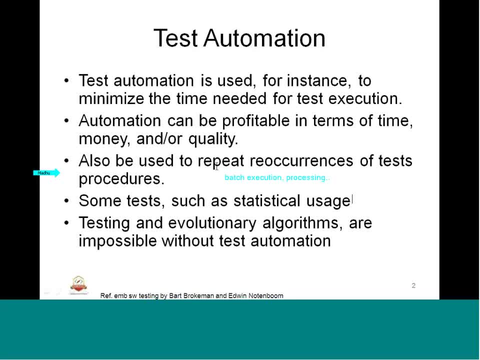 So the test automation is used in different situations where test that have to be repeated many times. the basic test with a huge range of inputs are there. the same steps have to be every time but with different data, Very complicated error phones test. that means we have a piece of software having more errors. 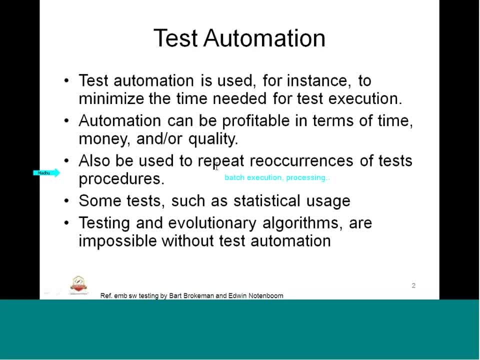 and all that and every time different errors are coming. so it is better to automate it so that the minimal human intervention is used for that. So this is very useful for complicated tests. but testing requires specialised equipment which will generate the appropriate input signals at the system and capture the output. 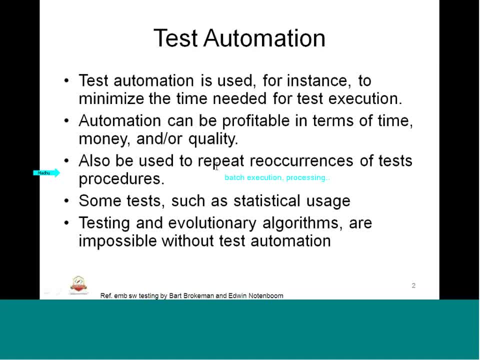 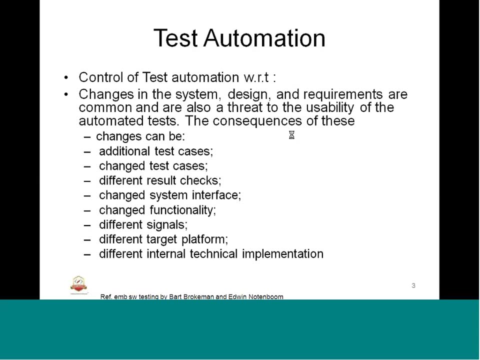 and analyze the output, unless this can be done manually or the tool itself can be used in terms of analyzing it. okay, So continuation of our test automation so we can have the control of our test automation in perspective. changes in the system, design and requirements are common and are also threat. 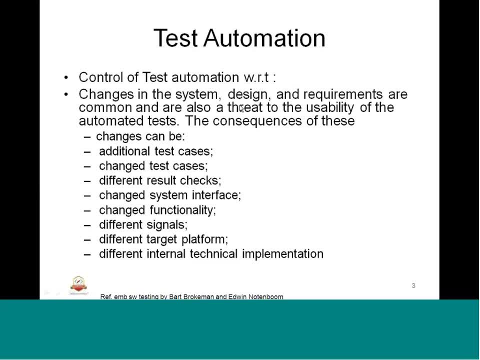 to the usability of the automated test. so what will happen is we have test automation completely for the requirements, sometimes the changes or the fixes that could happen to the system Or the tests that are going to be applied for the system. so the consequences of those 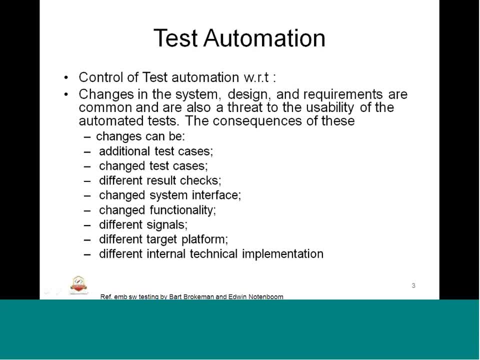 changes could be changes on test cases. additional test cases are available with the different aspects when different results checks are there and the framework has some impact in terms of modifying it. System interface has changed. there is a change in functionality, so signals have changed. 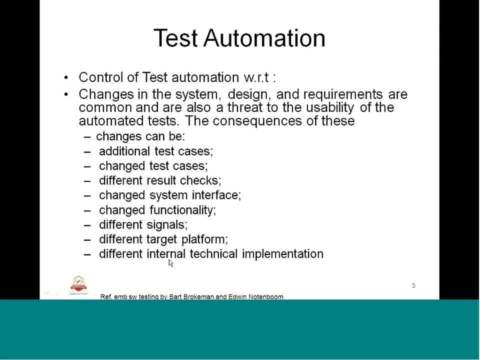 from one built to another built. there are different hardware boards, different version is being used, then there is a possibility that automation may fail or collapse. so control of the test automation is very important. we should have scalability of the test automation also. 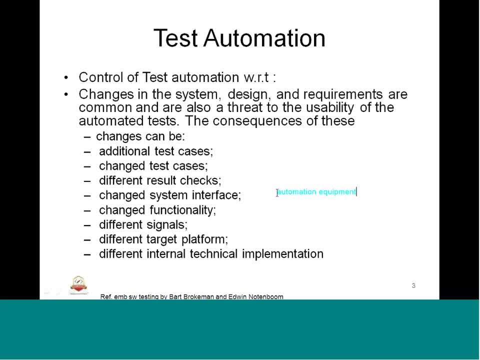 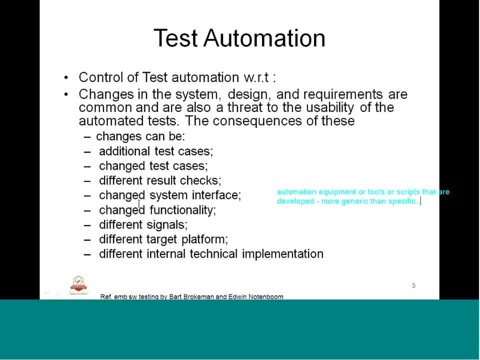 consequences of changes will have less impact on modifying the test automation. So basically, automated testing saves money and time and quality will be better because less human intervention is there. we are depending on the system and the tools of the framework, and the framework is stable. once you make it will, it is expected to behave same way. 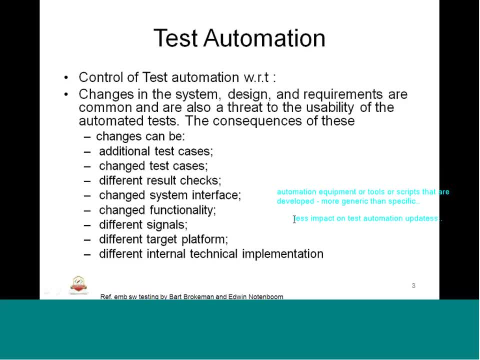 So in terms of injecting error by the user is very less and several times that can. test can be reproducible, so this is also very important. reproducibility of the test, execution, pass fails etc. is easier with the help of test automation. This means that the automated test should be used for consecutive releases or in different 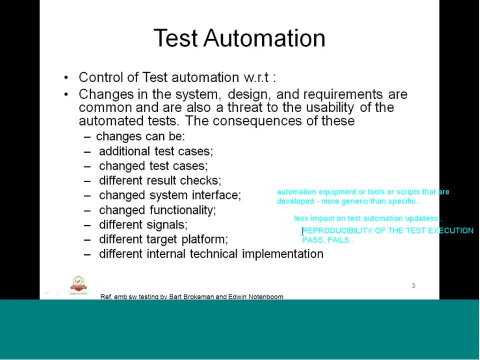 stages of development. that means the same sort of a automation should be able to use the different releases of the software build and the equipments. sorry, the embedded target could be So, which also means that automated tests have to be designed to deal with these uncertainties due to change in the system design. 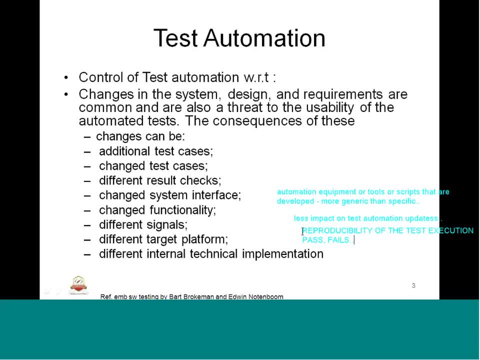 So we will see how automation test can be implemented technically in a net shell- basically we will try to understand that- and automation test basically being developed in house with the help of commercial tools basically that are available in the market. and of course those tools have to be foolproof and should be qualified, especially in the industries. 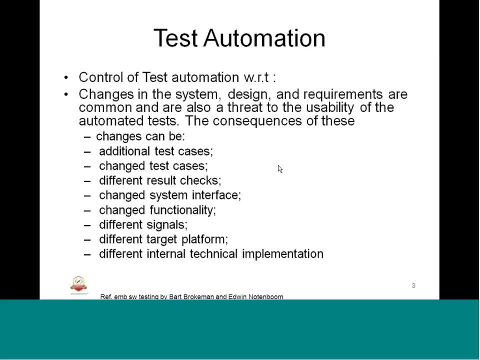 of automation, Automotive and aerospace is very important because it has to be reliable and we need to produce the consistent results all the time. So then also, we will study about how the process of introducing automatic testing and similar development process, such as requirement deployment and maintenance. 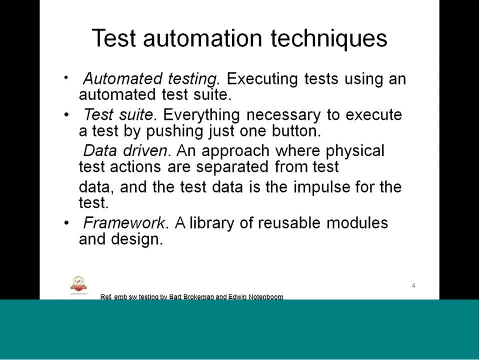 Okay so test automation techniques: automated testing, executing the test using an automated test suite. So there is a test suite that will be used which will be executed for testing the specific software piece, Test suite, everything necessary to execute a test by pushing just one button, ideally. 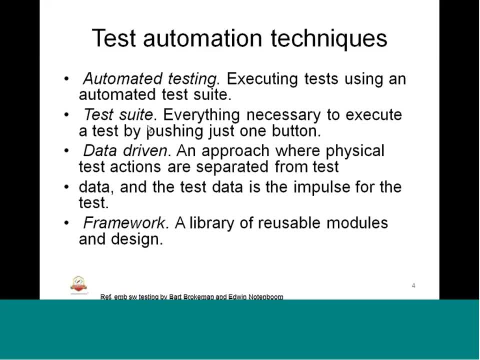 there should be that actually test suite will be triggered and it will take care of all controlling, picking the data, signals and driving values and data. So that is a test suite. So that is a test suite. So that is a test suite. Theという robot say can beہ. 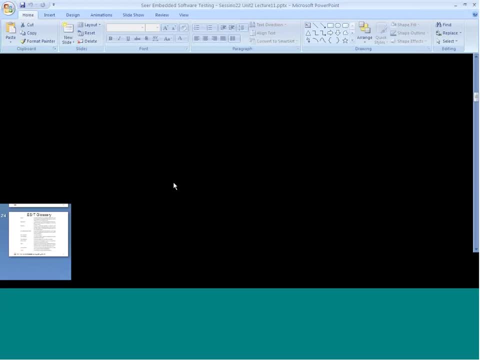 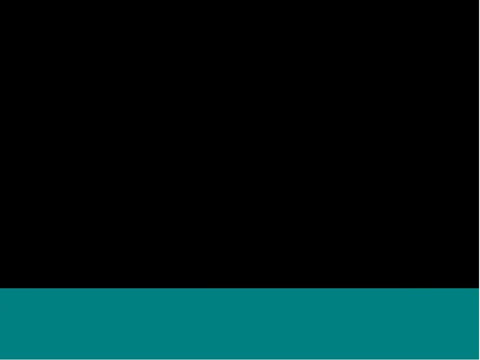 get such andere. Thank you, Thank you, Rohit, Thanks Rohit, Thank you, Rohit, and Dr Kes, minha husband Sw. fortunately we are now the end. So, to finish, we are going to set up The testing. our test be data driven and there should be a frame work in the end where a library of reusable 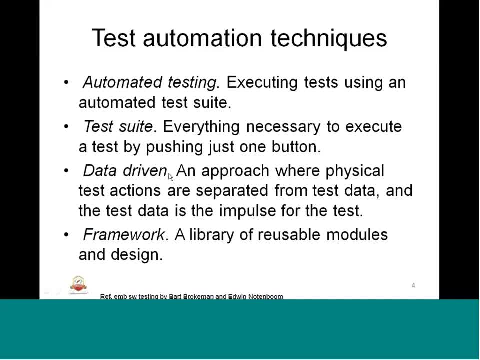 models and that means, as you see, the test hubs and drivers. they should be reusable for many parts of the system. So test hubs, test drivers and common templates, or it is, it could be a minimum sequences in especially, I have seen lab view and you can see that there are. 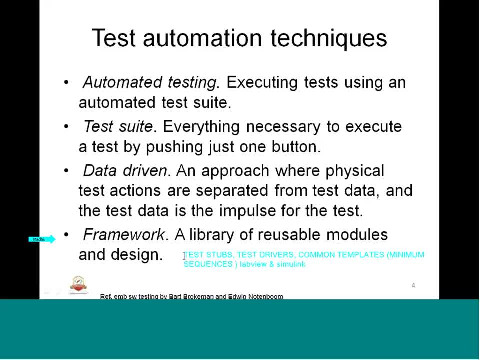 many similar link. it is very important: the sequences, the minimum templates. they develop it and they can use it as a plug and play for wherever they want to use it in the complete automated testing system. So there is a test suite. test suite will use this frame work. 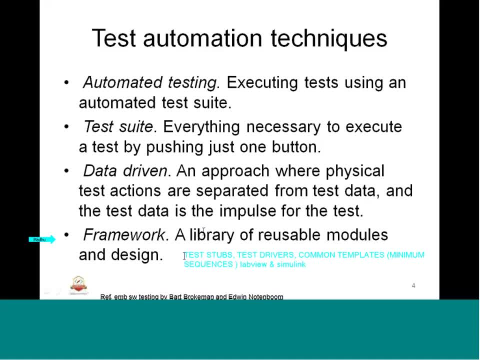 for the need of that particular test, So to maximize the maintainability, flexibility and ease of use. So some decisions: So to maximize the maintainability, flexibility and ease of use. So some decisions should be made to avoid a test suite from becoming where it is designed to be, as independent. 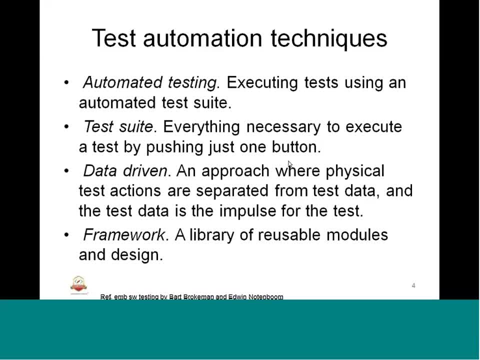 as possible of changes So that the frame work can be used. So it is very important to have a test suite and the system connectivity and the tests that are having data driven to be able to identify the approach for the underneath frame work. 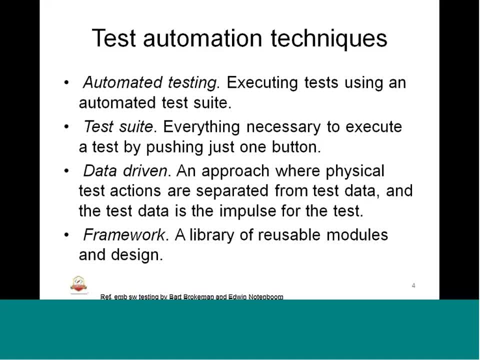 So generally the frame work is develop to avoid the huge dependency, So whether the dependency there it a minimum, as much as possible, So that the frame work is generally and the frame work can be use across to multiple functionality of the pieces of the software under the test. 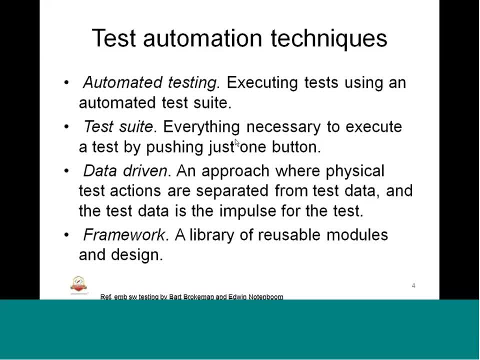 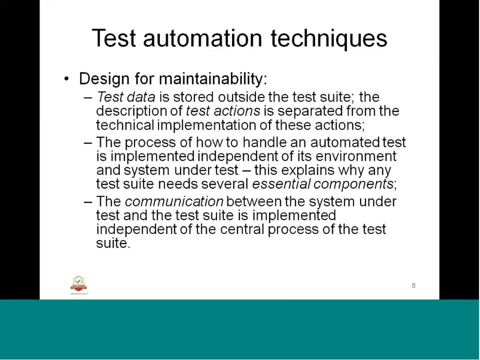 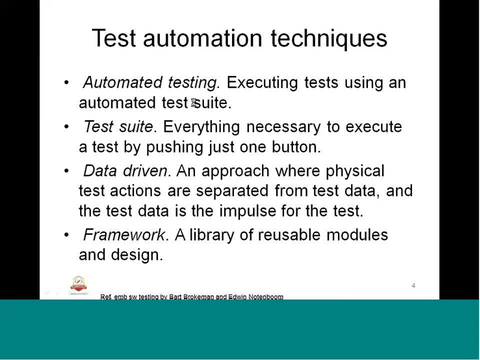 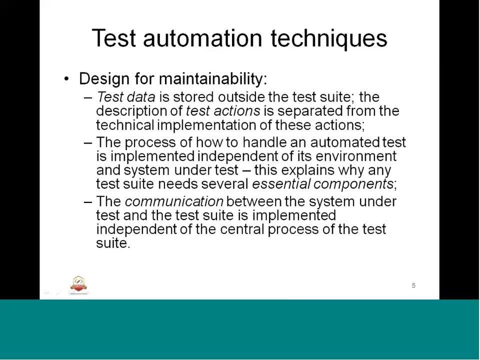 So that is the first step. Next is commercialised device. Okay, so design for maintainability. test data is stored in continuation of the test automation technique, We have a test suite data driven framework. then, for maintainability purposes, test data is stored outside the test suite. the description of the test actions is separated from the 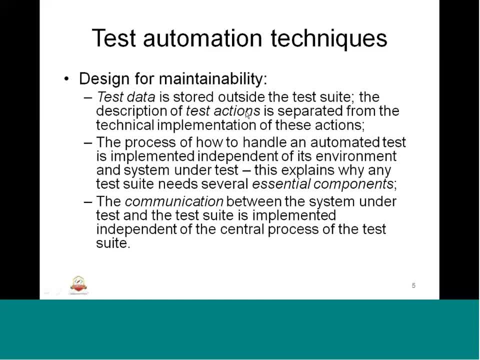 technical implementation of these actions. I will show you a diagram which is easy to understand. with the help of that, you can understand this description. A process of how to handle an automated test is implemented independent of its environment and system under test. this explains why any test suite needs several essential components. 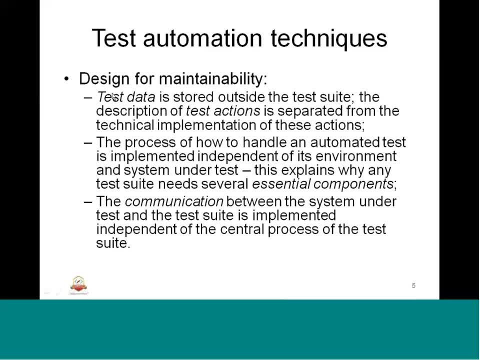 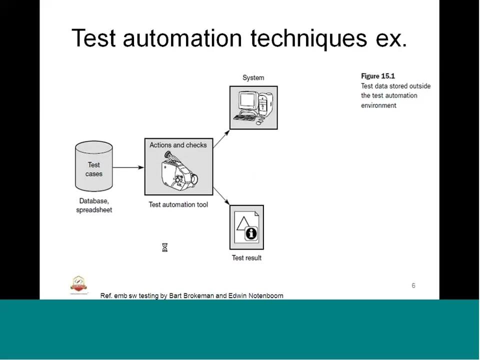 that essential components could be a test data and the framework and the test actions are inbuilt in the test suite. The communication between the system under test and the test suite is implemented independent of the central process of the test suite. You can see an example test automation environment how it is going to look like. so just a depiction. 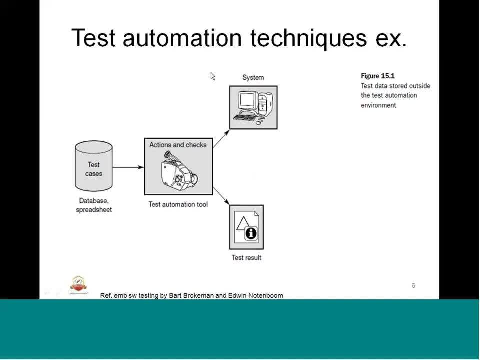 so it does not mean that the same thing is used in actual. the system that is going to be tested is here. We can see the system that is being used and we have a repository of test cases. In the test suite also, we have a repository of test cases. 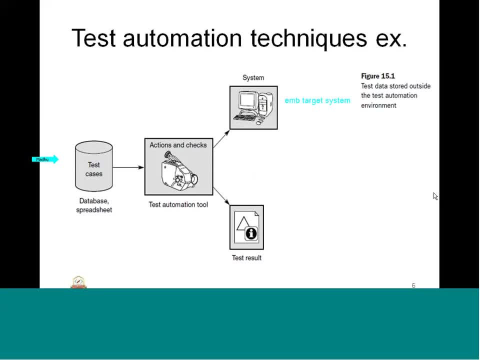 So in the test suite we have a repository of test cases. So when we are testing test cases, So the first thing that we do is toast test, we do test cases and we also describe in a simple way a sprint test. 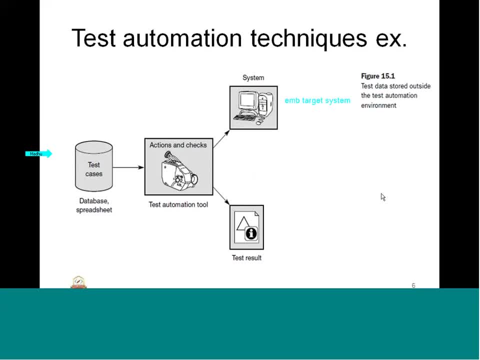 So all the test cases will have a database spreadsheet, whatever it is that will be picked by the automation tool to pick up that and it will run on the system and it will generate the result. basically, this is the flow where all the actions, checks, comparison, all will. 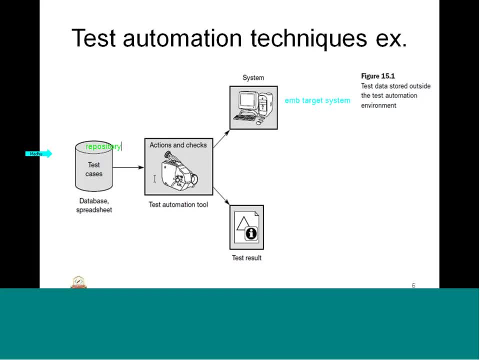 be done with the help of this test automation tool and the data is stored outside all the data, test cases, those things. So we know that the framework is part of this. this framework will pick up the test cases and it will apply the databases as the inputs and it will execute on the target here and 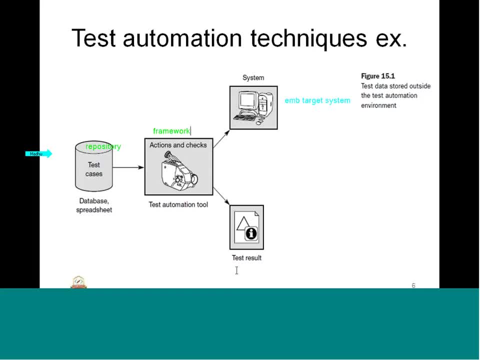 as a result of that, it will generate the report as a outcome of the test in a spreadsheet or excel sheet Or a text document or the logging, whatever is required. of course, also it will use the facility for the intricacies of the embedded systems, such as debuggers and all that, everything. 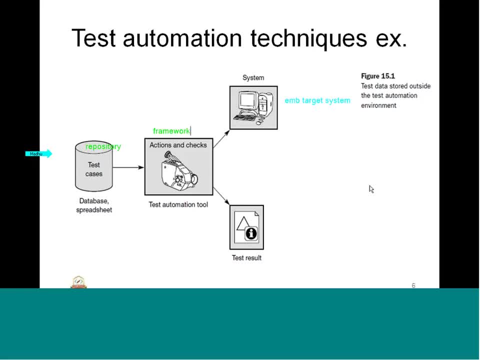 can be automated with the help of the automation tool. even the invoking of ID debuggers, analyzers, etc. Scope also can be triggered with the help of this automation. all this we need. we know that. So if you automate it, it will be easier for us to maintain and design the testing aspects. 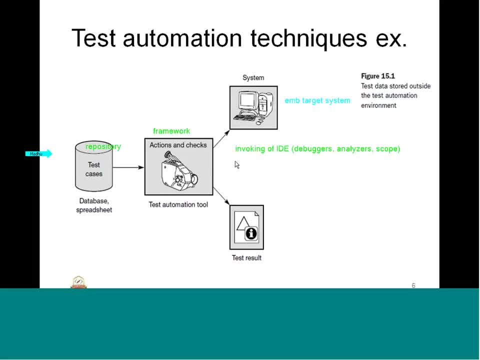 so that is how testing is done. this is particularly useful where we have a complex embedded software system. So another variant of: okay, so test cases are stored outside the test suite. So the test cases are stored outside the test suite. So the test cases are stored outside the test suite. 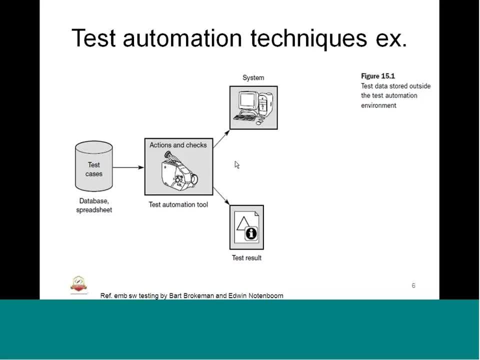 So the test cases are stored outside the test suite. How to say the test suite? yeah, they can store data based on the spreadsheet here, and additional test case means to the storage of the test case. So if there is any additional test case we want to do, we do not have to change anything. 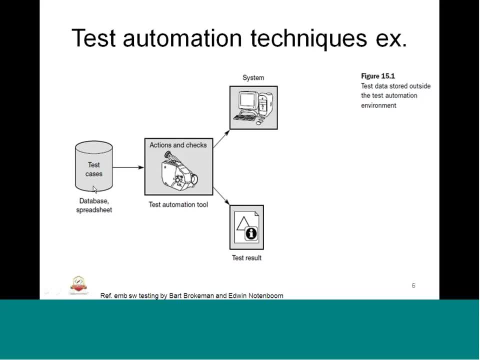 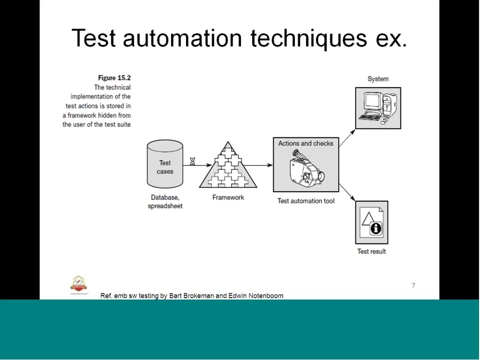 on this side. only you have to add the repository or delete or monitor whatever it is, So the test suite do not have to change, so the test suite will always be same. so another variant of this: this you can see in the next diagram where test actions and checks as part of the test. 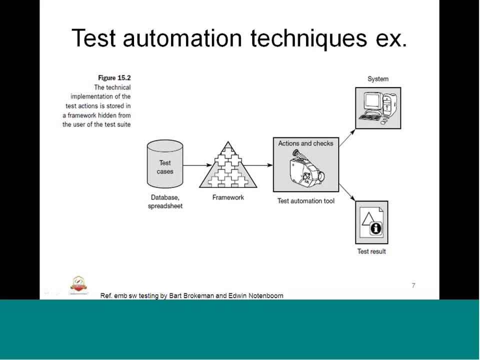 automation tool will work like a machine and the framework is outside. the framework is built little outside, with more automation here and the philosophy of test cases, data based on the left hand side in the repository, so the technical implementation of the test actions that are part of this are stored in the framework. you can see the blocks: these: 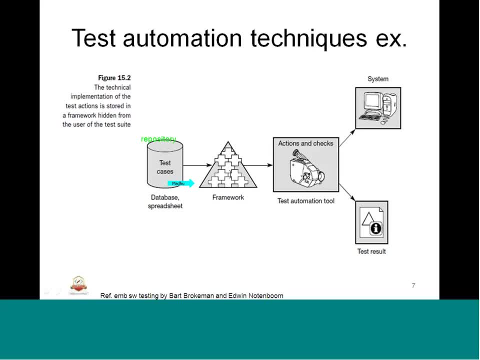 blocks can be a series of actions or the sequences, so that is given from the user of the test suit. so these are test suit. basically, again, the test suit will have a system trigger and specific test cases are picked up and the framework will drive what needs to be. 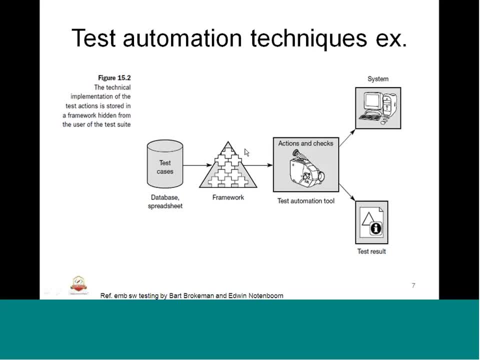 done so. that is the difference between this and US1, where we have the framework separated from the automation tool. of course, we can also call it as a test suit. Now let us talk about the independent automation tool. this bundle is very important here, where maximum automation is done with the help of framework and the action specific the tool. 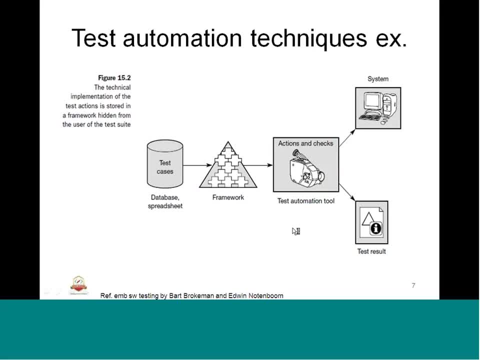 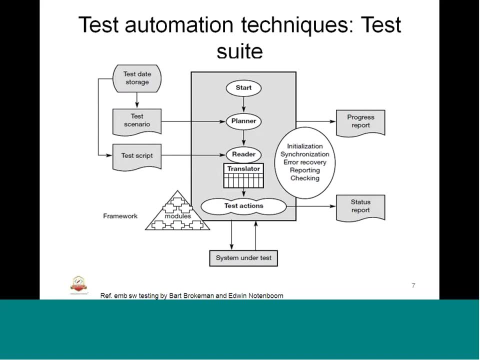 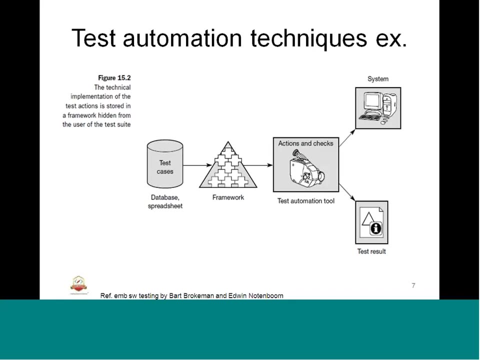 this tool could be lab, you test and or some link. there are multiple tools available in the market, so, basically, the technical implementation of certain test action can be rather complicated, so this implementation should be hidden from the normal user. you do not have to bother about where it is available, so only thing to know is which test actions are available. 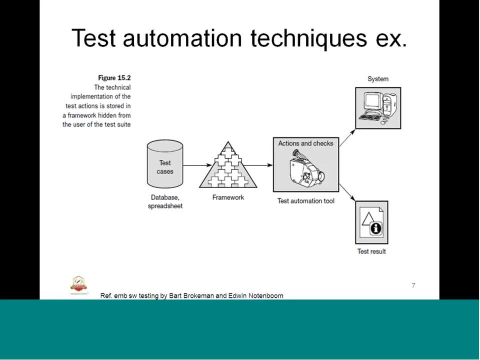 so those actions are a part of the automation. So automation will pick from the framework. so if the functionality of the system or test space is same but the technical implementation is changed- suppose we have a different implementation altogether on the embedded systems- the framework will modify. so we will try to modify the automation. 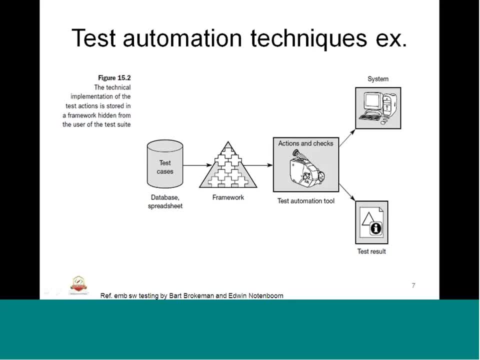 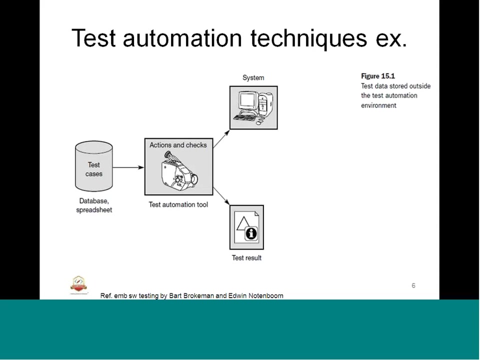 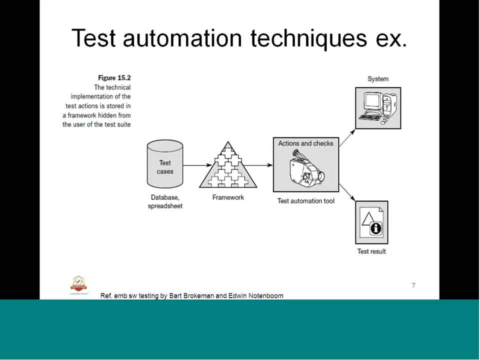 so in that aspect will be useful. so, for example, an additional interface is lagged or the signals have changed indirectly. So this is very important. Thank you, For It is. the main point is that you have to know the köpütü, okay. 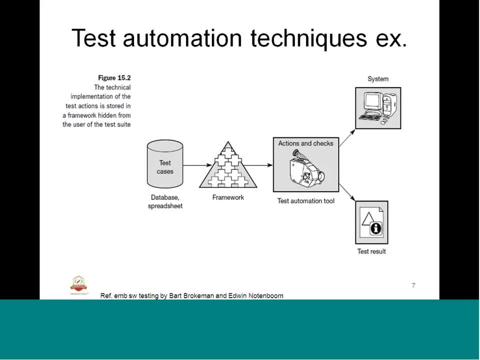 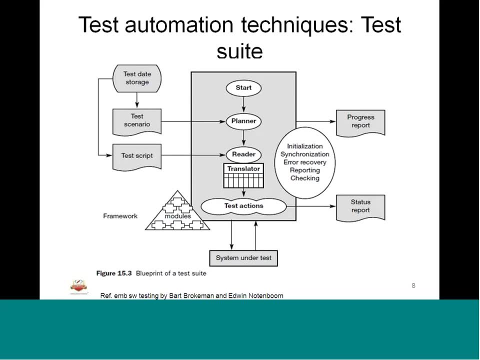 Okay, next one is the test suit: how it looks like, the intricacies of the test suit, basically, it is also called in the book. it is specified by made of a testing by Bart Brockman and Edwin notebook. I am referring most of the pieces there because that is a more relevant. 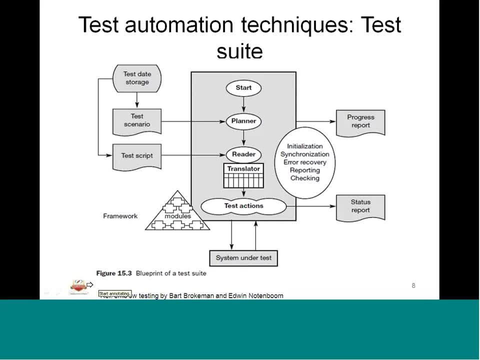 but I see you can refer this book online and the suit has several components inbuilt, so let us see how it flows. so this is the basic. what is that called on? framework having different models? you can see it here and it has a flow. there is a start, there is a planner. 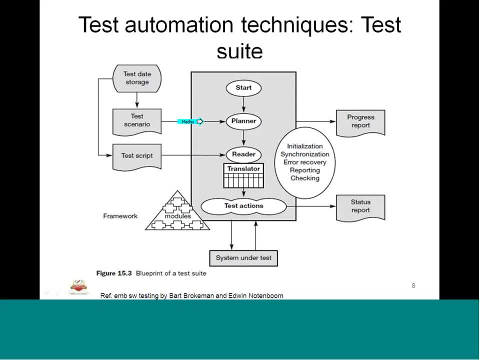 there is a reader, the planner will pick up a particular test scenario and you can see the scenario from the test data storage. that means we have a test data storage in terms of a database having signals, its definitions involved and the cases, also test cases also specifying the test scenario, and that scenario will be picked up by the planner module. and 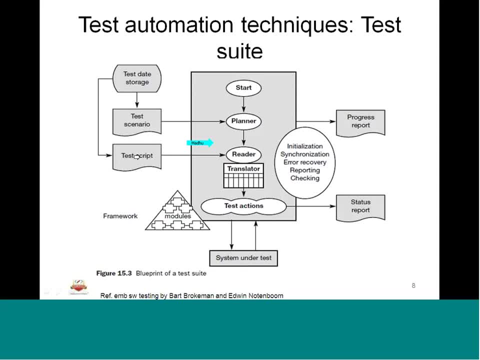 the next one will be reader for that particular scenario. the particular test script will be read from the stored database or the contents, And there is a translator. the translator could be applying this into the understandable actions on to the target, so the test actions are derived from the translator as the intermediate. 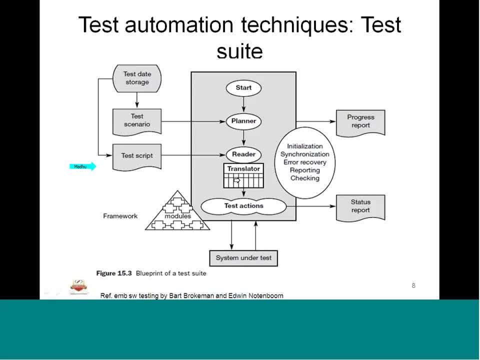 layer. so the name is translator, but it could be anything. when it comes to the actual embedded software testing automation, different names could be used. so the actions could be initialization, synchronization, auditory report, Checking and all that part of this framework having different modules and, as a result of 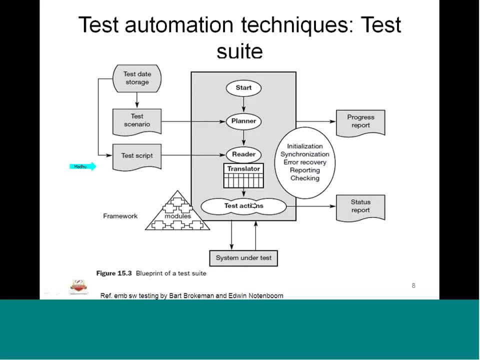 test actions. we have the status report and the actions will be applied on the target system system under test and the status report will tell that, for each of the script and the scenario, what is the pass fail value or the what are the passes and where it has failed. 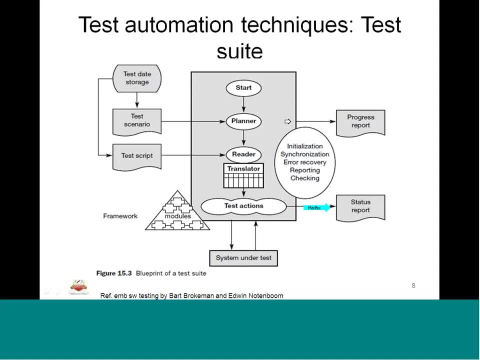 And also when we do the batch run, we can get the progress report in terms of pass fail count. it is called pass fail count one down progress. it is basically a chart of the entire test suit or the bundle of the test suit: progress. so that is how we use the test suit in terms 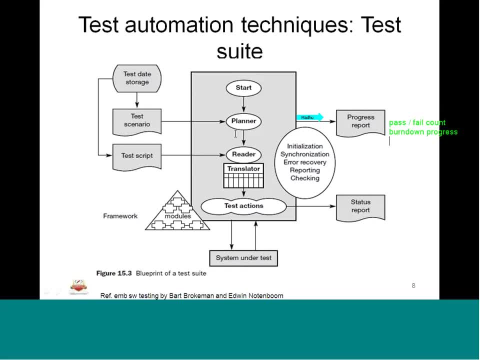 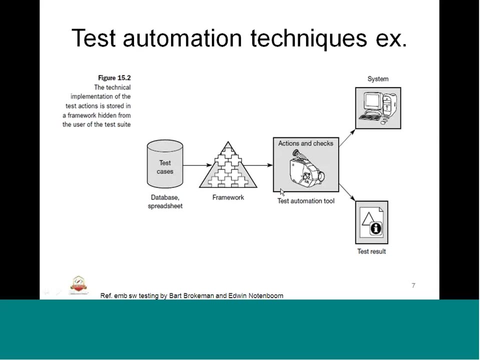 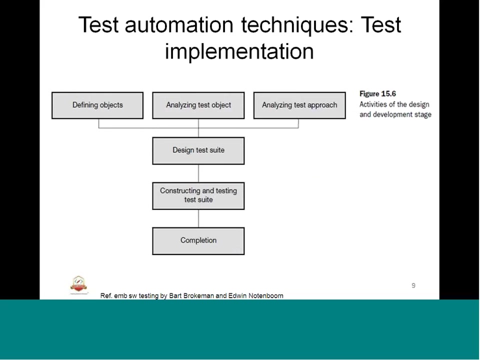 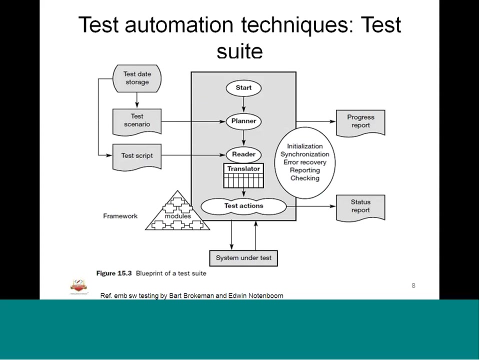 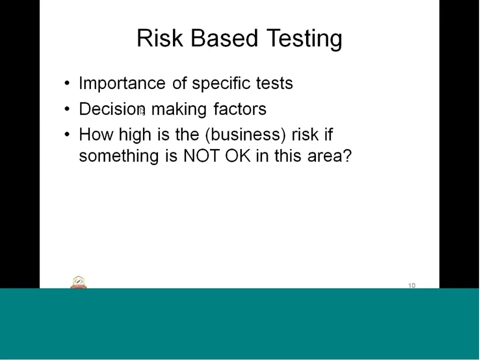 of automation. So that is about the testers or the test development team to have what sort of a approach for different blocks of the underneath embedded system. all this will be part of the implementation. okay, so that is about the test automation technique. The next one is we will study about risk based testing. so what is the risk based testing? 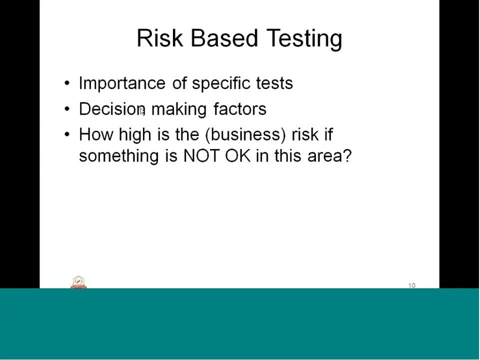 and why it is needed and some of the embedded systems they used as an important testing. So basically, in a structure test approach, this is very important and it contributes to a more manageable test process. priorities must be set and decisions made about what. 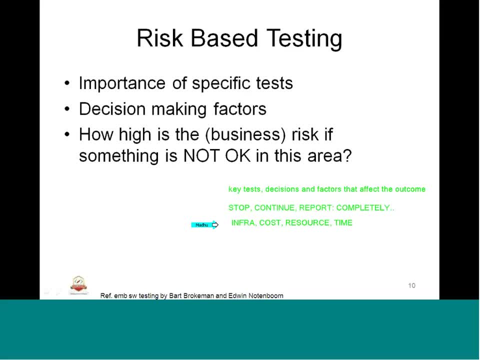 is important and what is not, is all being specified, Okay, so important means what it is- very subjective concept, of course, with a risk based strategy. evaluating the importance is about answering the question something like: how high is the business risk if something is not okay in this test? that means, if something does not. 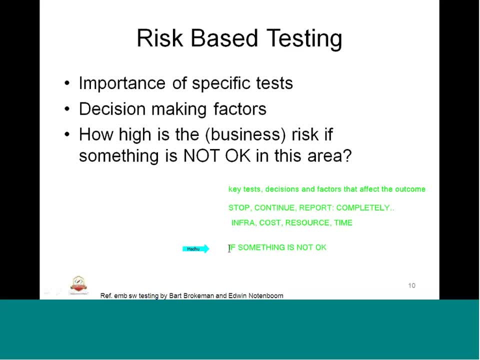 work while doing the testing. so what is the impact of that? what is the importance of being that as not okay? so all answers for that will be part of the risk based testing and that should be communicated. so we need to define it. 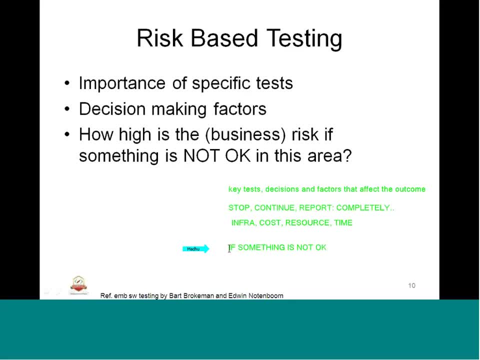 So basically, risk is defined as the chance of failure occurred or occurring related to the damage expected when it does occur. so what is the damage that is going to cause for that particular failure? so if the system is of insufficient quality, this may imply high damage to the product. for instance, it could cause loss of market share. the company 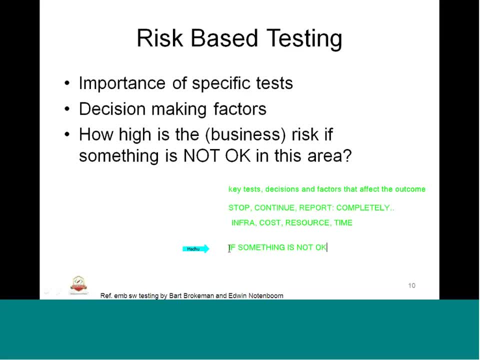 it can be obliged to call back millions of sold products. you have seen there is a call back of Toyota cars for a small issue that they found near the break. To replace that they have to call back, it is called as call back millions of cars. so 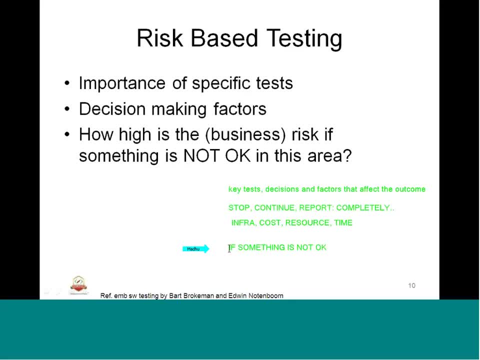 it is going to be a huge cost. so those will be identified while doing the strategy of certain aspects. so in that aspects, the importance of those key elements will be identified. that is called risk based testing. that will be under tests. therefore, the situation forms: 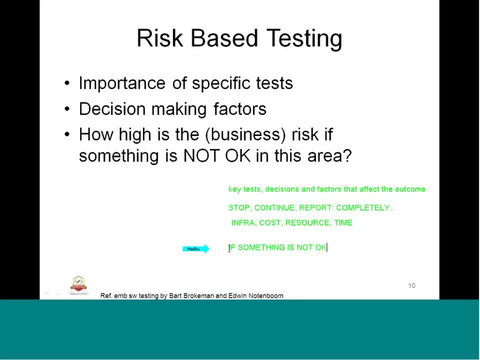 a risk for the organization, The highlighted elements which are called as a risk. so testing of those aspects will cover such risks by providing insight into the extent to which the system meets the quality demands. so if certain areas or aspects of the system imply high risks for the product, 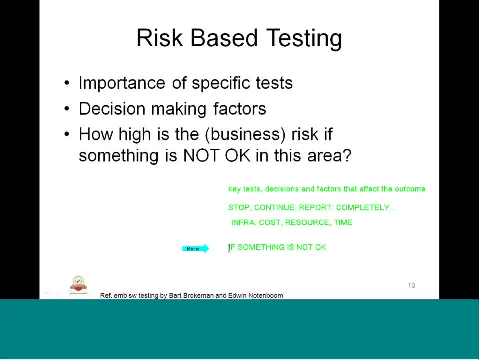 and more thorough testing is obviously a solution. So thorough testing of that particular aspects are the important parts of the system- needs to be done. so those will be done from the quality standpoint. Of course, the other way also is true. where there is no risk is involved, we may have to. 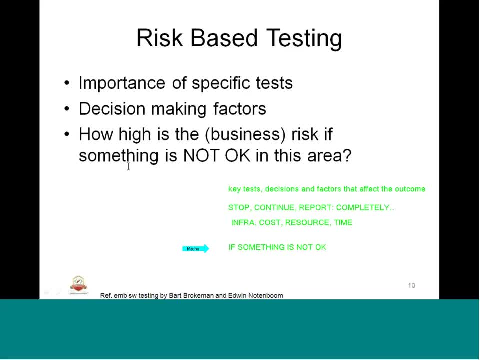 have a small piece of a test or if there is no test is required. we do not have to do a test when there is no risk at all. So how do we evaluate that no risk is involved or risk is involved, or if it is important or not important? so this risk based testing strategy probably will answer that. 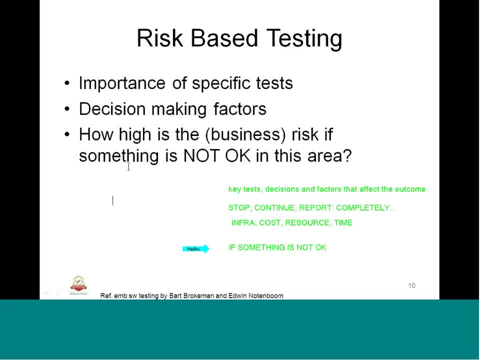 The attributes should be from the quality or the performance or the product outcome in terms of business objectives. so usability and all that will be part of this risk based testing strategy And the subsystems also could be commander based strategy. we have a big system having 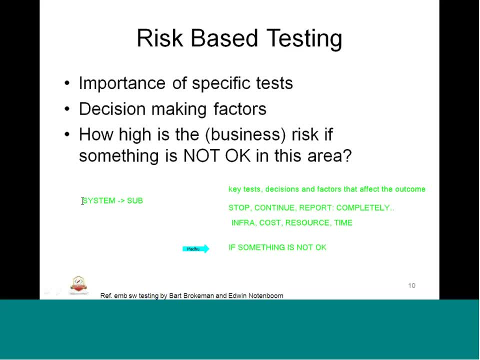 subsystem 1, 2, etc. all this will be considered for failure attributes and the risks and the importance of that. particular failures And how they do is Decomposition of the architecture, the high level information system. with the help of that they will arrive at the strategy decisions. 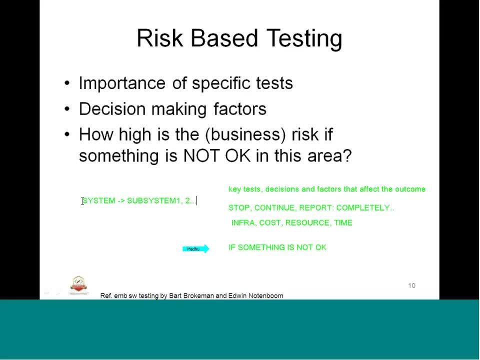 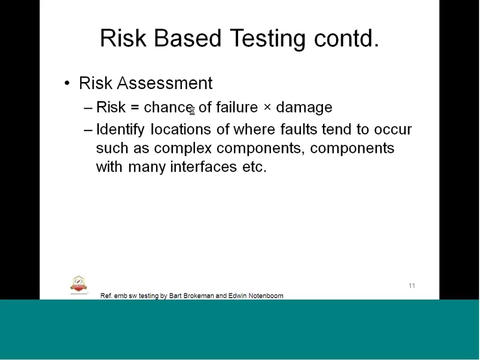 This specifically done in with the help of quality attributes such as ISO 9166 and DO also, they applied, So it is very important to have a decisions making That is for so such important aspects of the system. okay, So that is what is called as a risk based testing. risk assessment has to be done for the identified 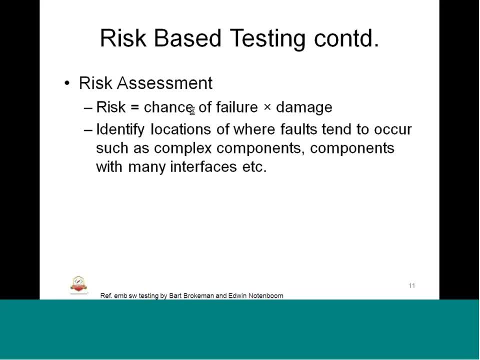 risks, So chance of failure into the damage is going to have, is what is called as a risk and that will identify the risk. Okay, Thank you. Okay, Does thatricity test in the particular test strategy for type of risks that are identified? 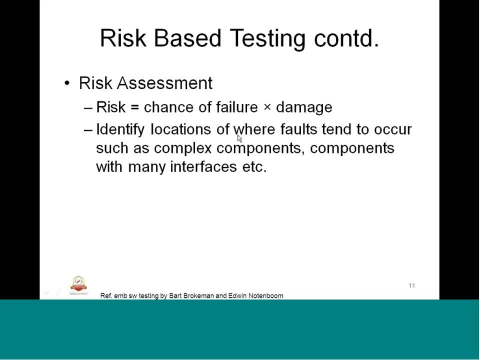 So identify locations of where the falls can occur, such as complex components, compounds with many intraceratops signals, etc. Those need to be identified first, and identification of what are the chance of failure and what is the cost of the damage, So that will be arrived with the help of that risk, will be assessed. 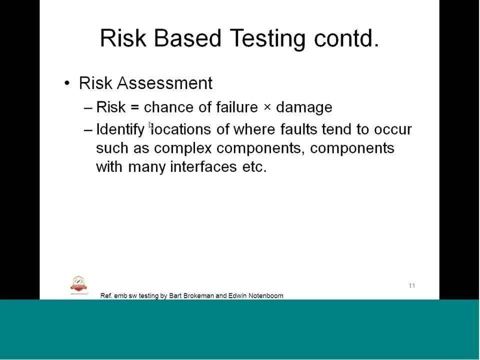 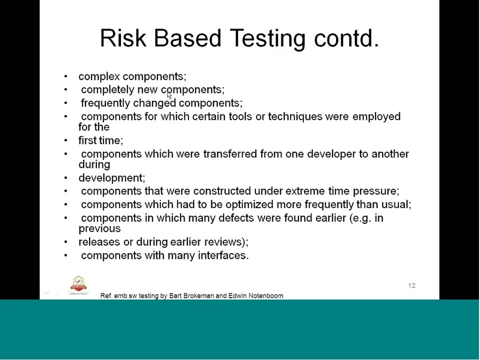 So that is called as risk assessment. important part of the risk based testing And identification could be on some of these things like complex components, completely new components, if the people are not knowledgeable, or if it is a new subsystem that has come to market and that is getting used. that is the risk, and if the component is getting changed, 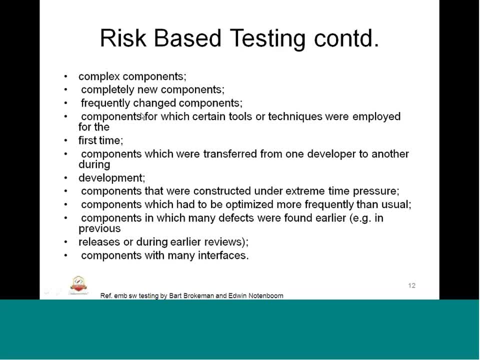 again and again in the world or in the embedded system could be embedded software. it could be- and that is also a risk- Components for which certain tools or techniques were employed for the first time and components which were transferred from one developer to another developer during the development. 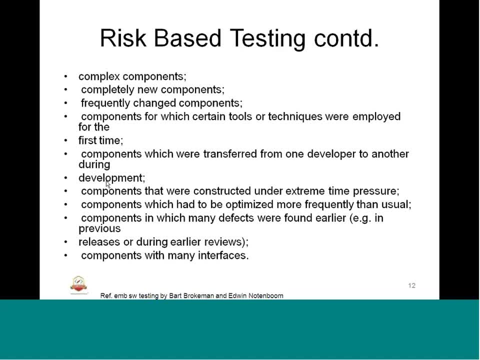 there is a chance that the new developer would have injected some values Components that were constructed under extreme time pressure. It is a very important term because what happens in embedded software development? there is a chance that the last minute work will be more and due to delays in inputs for the 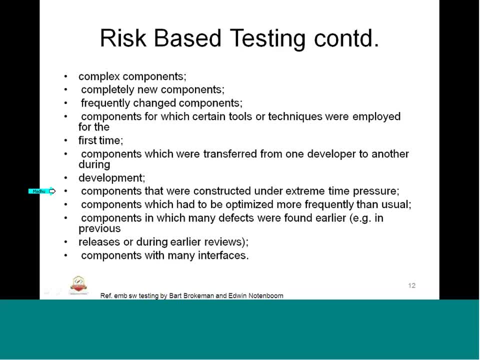 developer or the tester. due to high pressure, time pressure and time to market, the chances of injecting the values are more, And those components need to be identified as components. Thank you, Thank you. This is the last part of the introduction of embedded software, but I would like to 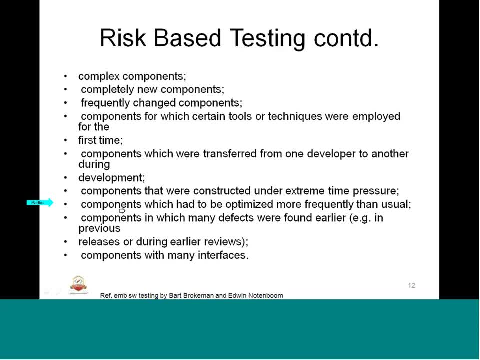 share some more information about the embedded software. So components are not only hardware components but also some kind of hardware components. So there can be a lot of hardware components, and here component means it is not the hardware component, It is any piece of the embedded software system. 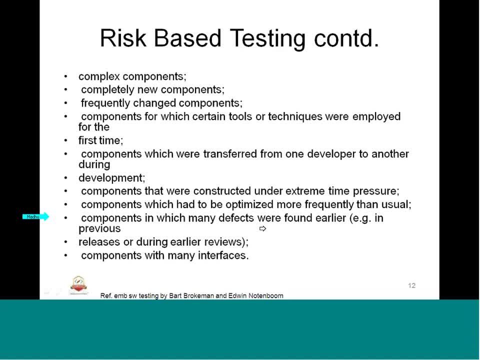 So components which had to be optimized more frequently than usual. that means more optimization is required on those components that also can come under risk, Components in which many defects were found earlier. during earlier reviews we saw that certain components are having high defects still that 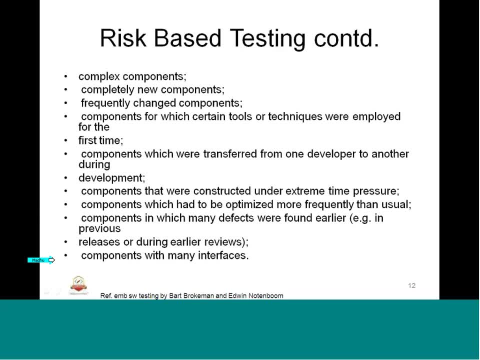 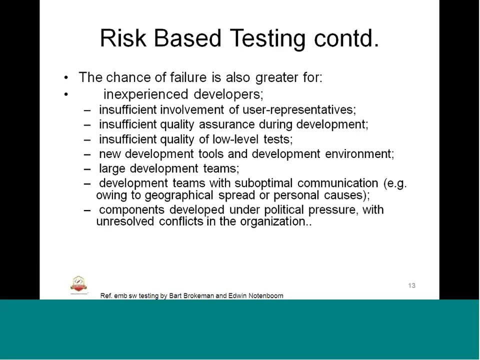 has a high risk. components with many interfaces, many signals are being used in that components. that is also a risk element, So the chance of failure is also greater for the inexperienced developers. insufficient involvement of user representatives, insufficient quality assurance in development, insufficient quality of low level test, new development tools and new development environment also. 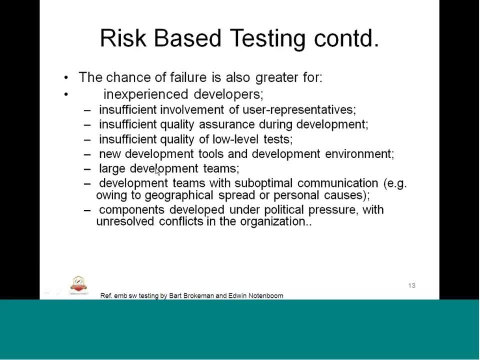 is a risk. large development teams where segregation is very difficult and interaction of different teams also is a risk. development teams with suboptimal communication. example, going to geographical spread, That means the development teams are not able to do that, So the chance of failure is also greater. for the inexperienced developers: insufficient. 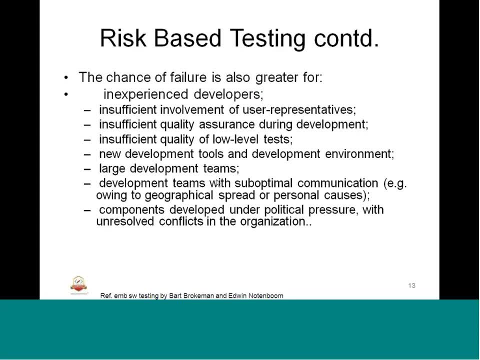 computing for reason. So what happens in the next 12 months? we have seen emirate industries, that説 across geographically different locations, such as in aerospace industry we develop the entire system. or example, at Boeing, it is done in Seattle, USA, whereas development is done in a different location, in fuand. 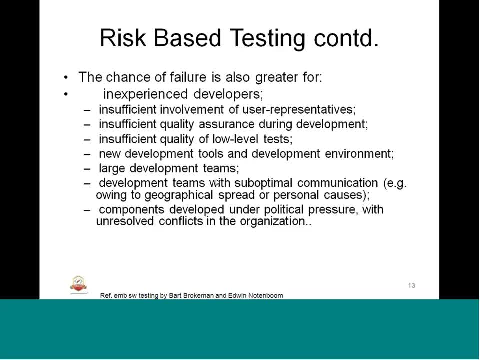 testing is done in India and fabrication and assembly is done in K Characterise 0. Thermo. so development team for testing team iscciones completely, providers andulsion disintegrated and interaction have to be done efficiently. so as long as that is there, the 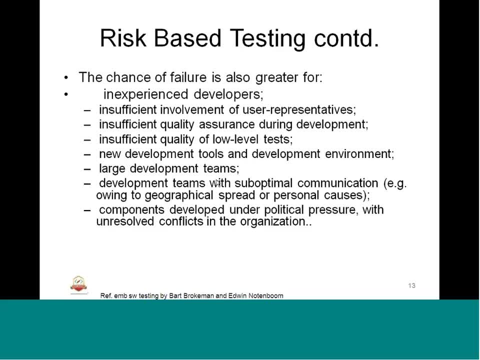 chances of failures are more, due to which there could be slack in some of the coming to form or convincing the facts. so there will be some hidden issues or errors. that system can have components developed under political pressure with unresolved conflicts in the organization, or shufflement in a team also could be a fact of risk. basically okay. 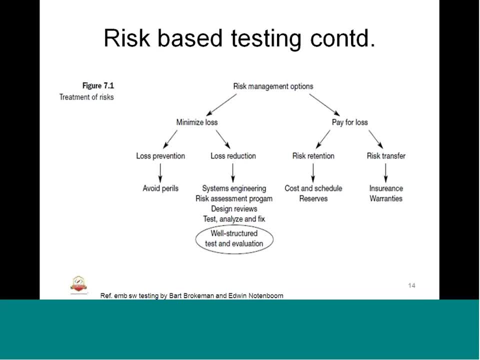 So that is about the risk based testing. we come to the slide where, how we can treat the risks, there is a term called risk mitigation. I think it is all management aspects. we will study in details but at least for understanding sake we will try to go through risk mitigation. 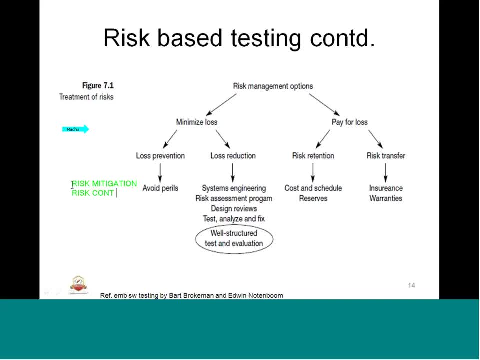 and risk. contingency means we anticipate the risk and we will work out what best we can do. in the contingency and risk mitigation is, if the risk occurs, what would be our approach? so it is part of the risk management, Thank you. So what are the options that are available? so categorization is something like this: 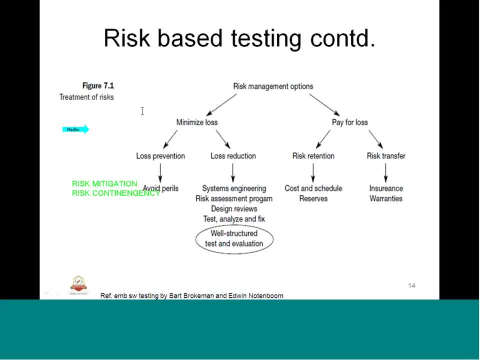 So the required information for risk assessment is easily obtained from different sources and with the help of those sources We will arrive at different risk management options. So we have a broader categorization as minimize loss or pay for loss. so here again the complexity. 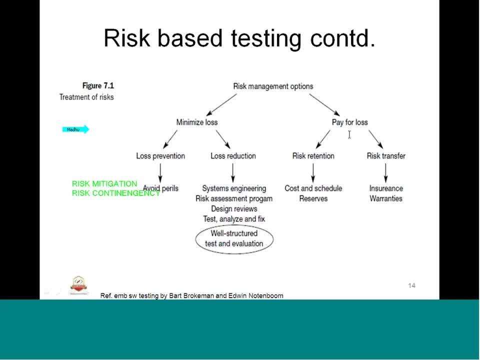 which matters. based on that the risk options are derived. Okay, so minimize loss is what is one category of treatment of the risk where the loss prevention and loss reduction and any threats we have will be done with the help of certain mitigation plan so that will work out for the loss prevention and in loss reduction system engineering risk. 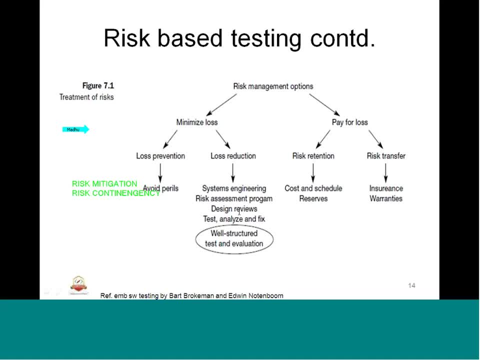 assessment program. Okay, So use, test, analyze and fix well structured test and evaluation. so all this will be part of the loss reduction. so we are going to have a loss or certain failures. all we can reduce it. So these are all the aspects which can be treated for reducing the risk and as we progress, 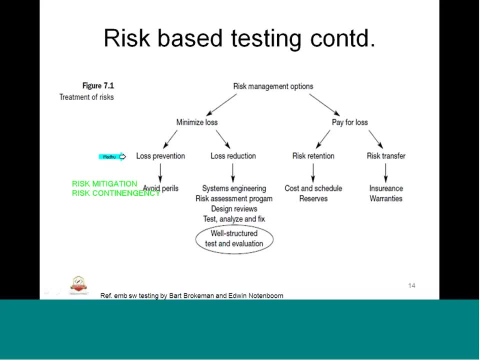 towards embedded software testing. we should try to reduce the risks- So loss of loss prevention- and try to avoid the threats that are there for the particular system. So this is only one path where we are trying to minimize the loss. and already the loss has occurred and the failures are there. risk is realized. then we have to pay for the loss. 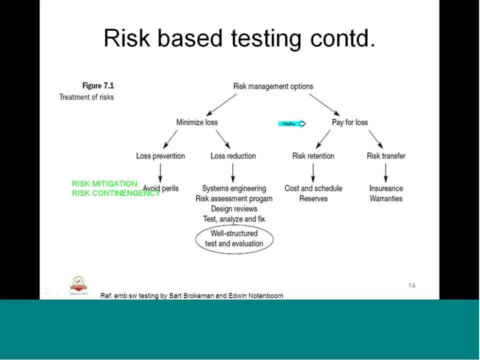 so how are we going to re risk it or treat it so? risk retention, cost and schedule reserves. that means we have a reserved cost for that. we are going to retain that risk and we are going to pay for it, or we are going to transfer that risk so that somebody else can continue. 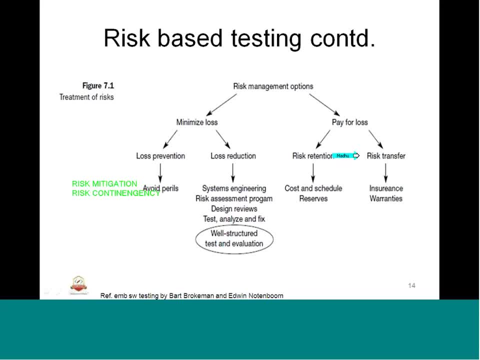 on. so this is basically a management thing and if that is coming under warranty and all that as part of that, it is taken care. so risks are very high. element important thing in the embedded software testing as a management aspect that need to be mitigated and continued. 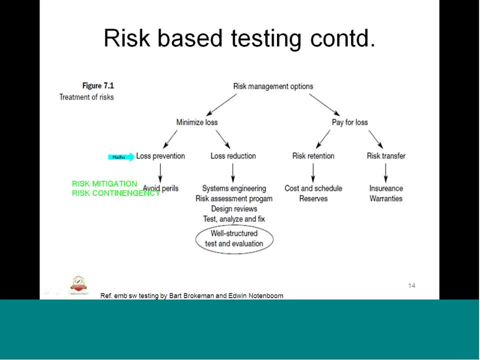 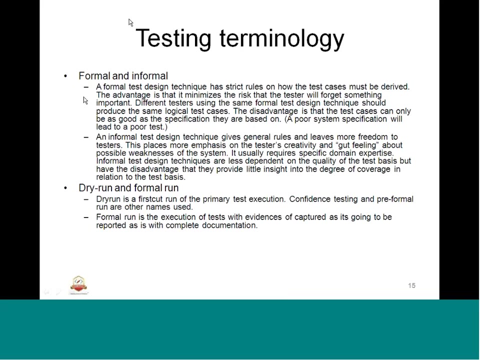 So that is about risk based testing and risk based testing aspects and test strategy, and we have a couple of important things that is used in embedded software testing method. that is called formal and informal testing. so what is the formal and what is informal? and the other aspect is the testing. 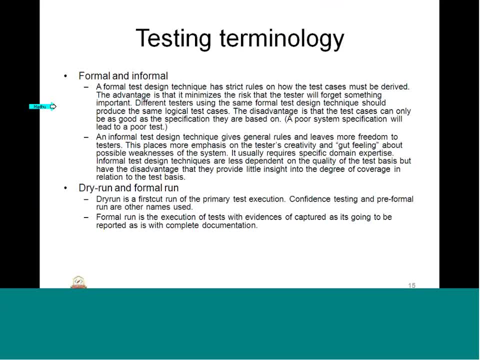 So the formal testing is dry run and formal run. okay, so these two are being used again and again in the software industry. we will try to understand what is formal, what is informal. if formal test design technique has strict rules on how the test cases must be arrived. 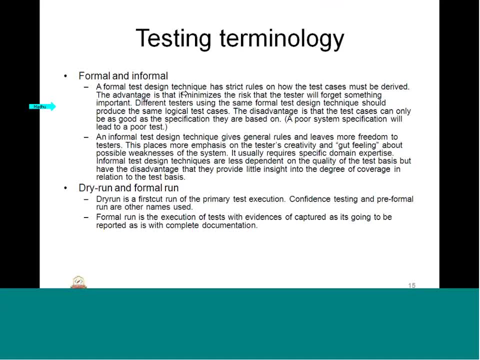 documented or a process oriented rules that will be documented, reported and frozen so strictly. we are going to follow that In formal test design technique and execution. the advantage is that it minimizes the risk that the tester will forget something important, and all because everything is based on a laid 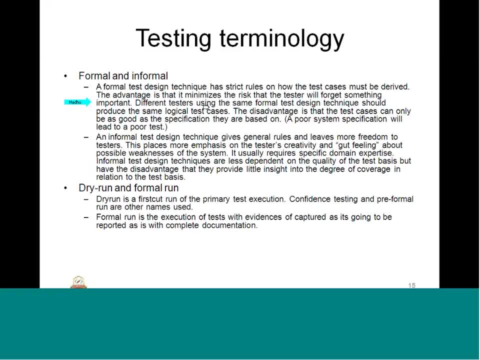 out process, so different testers using the same formal test design technique should produce the same logical test. that means we have a chain or the cycle that is well defined, so the user will follow that and we do not have to bother anything out for that. Thank you. 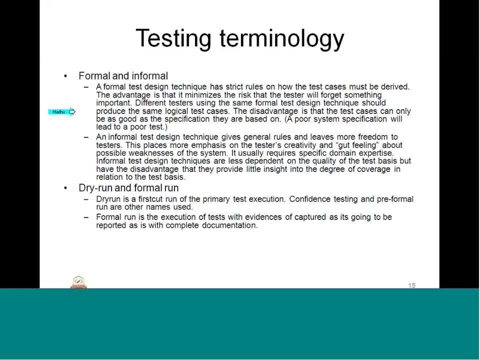 So testers will use the same formal method or the design technique again and again for doing the test and producing the results. The disadvantage is that the test cases can only be as good as the specification they are based on. a poor system specification will lead to a poor test, because we have already 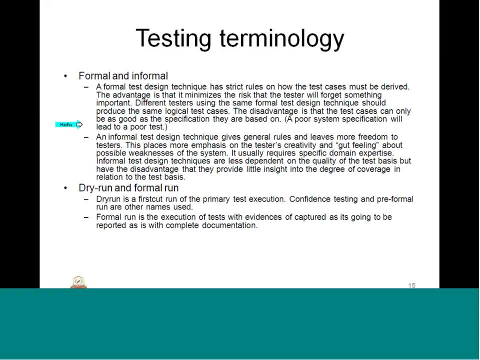 committed to doing the test and we do not have any second chance for revisiting the specification or the test design. So we have already committed to doing the test and we do not have any second chance for revisiting the specification. that means we have only �J эк sink gear to do it. 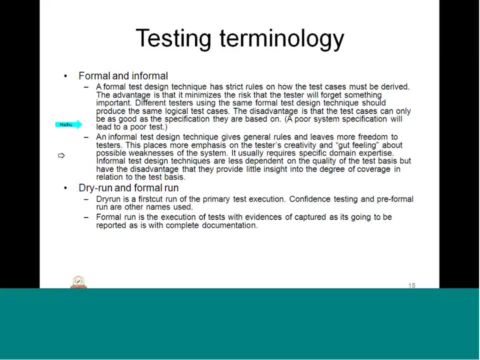 So, of course, if it easily fails, if it is going to happen, it is going to happen. and informal test is the another one. we said design technique that gives the general rules and leaves more peep to the tests. that means informal test. the tester has a second chance of revisiting. 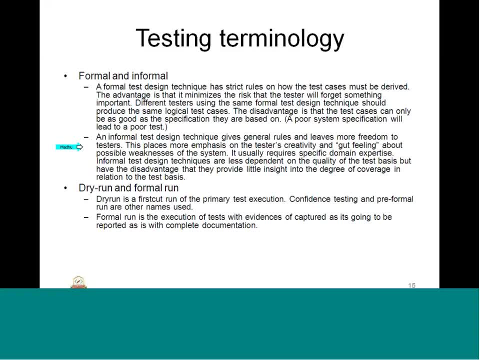 technique and he can slightly modify or there is a scope for improvement. there are hooks where he can add new techniques or smaller sections of the scale of the web to design content and other things, can adopt some changes or propose some changes. there are what is that called templates, where 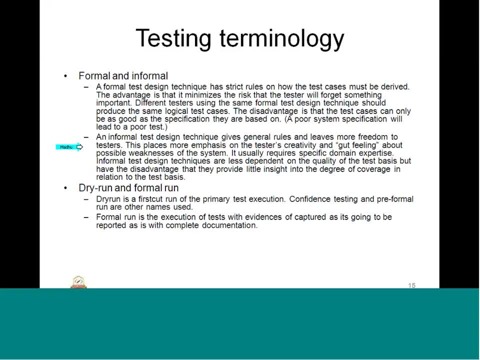 he can provide proposals to modify it and still there is a chance that he can improve the product before the product is out for delivery. So this places more emphasis on the testers, creativity and that feeling about the possible weakness of the system. that means the tester will have a full confidence of the embedded 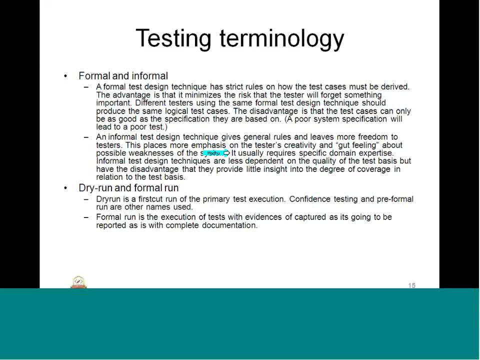 software system. It usually requires specific domain expertise. as I said very much, it is important to have a system knowledge of the domain. here domain means it is not just about the product and the product line Where it is being used. the product could be used in certain avionics, subsystems or systems. 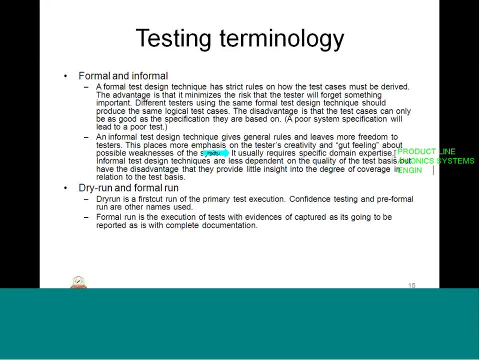 it could be used in Indian types, could be used in weather forecast, it could be used in breaking, because breaking many, many, some small subsystems. So that is the main thing, Okay. So we have test. what we are doing could be part of that underneath that, and we have telecom. 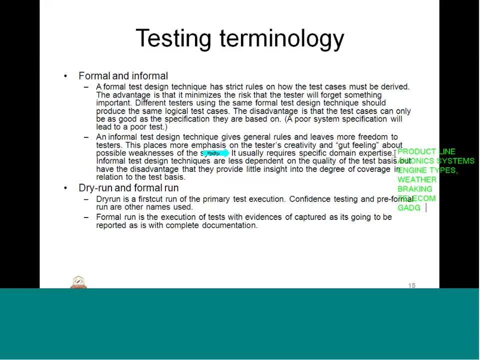 we have gadgets such as home entertainment or set up box, whatever it could be. So all this will be requiring to have a thorough knowledge of the domain of that particular embedded series where the product is being developed, tested and deployed. Okay, So informal test design techniques are less dependent on the quality of the test basis. 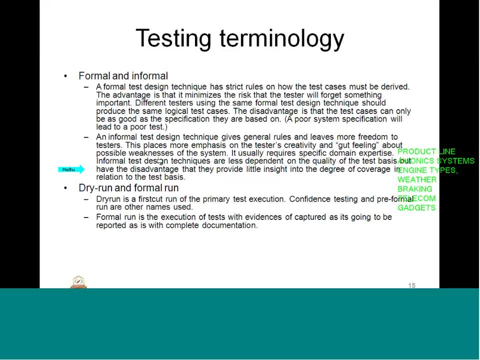 but have the disadvantage that they provide a little insight into the degree of coverage in relation to that test basis. that means everything will be informal, the coverage we cannot take the credit test and it is outcome Okay, Thank you Then will be coming simply because so whatever that the test has done in the informal testing, 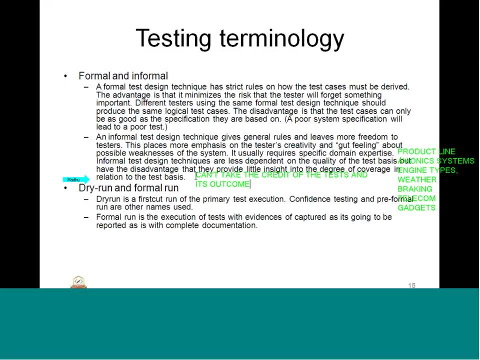 is all intermediate: once crozon, once our final, once. So that is where it has a disarvantage. but it is advised to have an informal test before we start the. The flow should be something like: we begin with informal test, identify all the, get a. 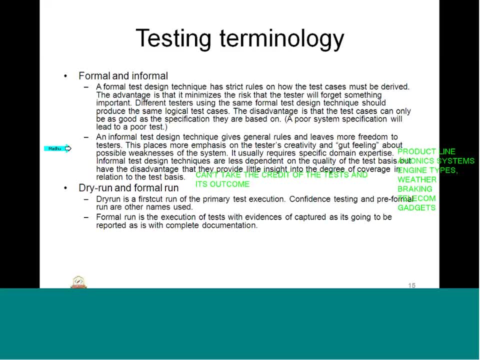 good confidence on the entire system: understand the domain, apply the techniques, improve the techniques, optimize it and anything that we want to do before actually the formal test. So they use it in the ML system: industry formal and informal, these two terms is equivalent. 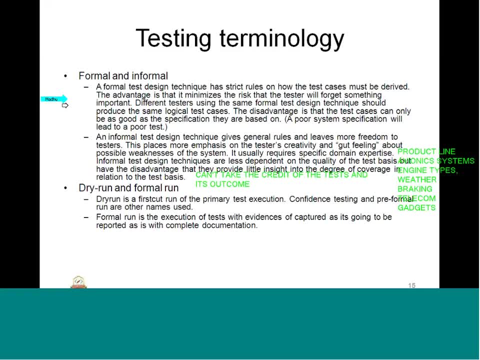 of that are being used in specific industries. that is called try run and formal run. The informal one is called as a try run. that is the first cut run of the primary test execution. so basically it gives a confidence And any revisit is required. fine tuning is required. all will be done with the help of 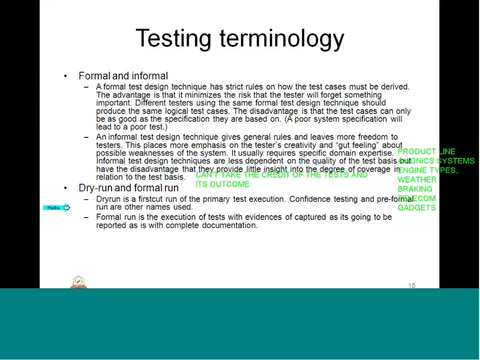 this try run. it is something like a informal or pre formal run and there are different names that are used, but generally in the ML industry they use it as try run and formal run. we know it is same as whatever we have studied in the previous bullet. 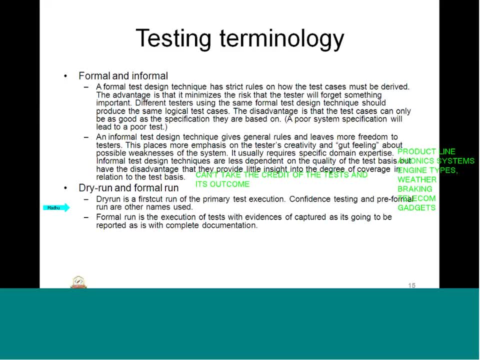 Formal run is the execution of test with evidences captured, as it is going to be reported with the complete documentation. So once we are done with this formal run, that is what is going to matter in terms of reporting: pass, fail, revisit, whatever it is required. 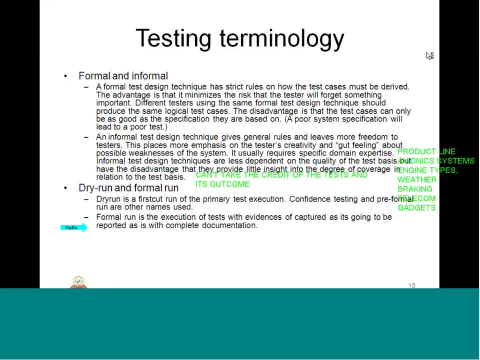 So that is about the ST terminology used in the ML industry, called formal and informal and try run and formal run. So with that we come to an end of our presentation, Thank you. So we have come to the end of unit one, so probably we will touch base. what are the chapters we? 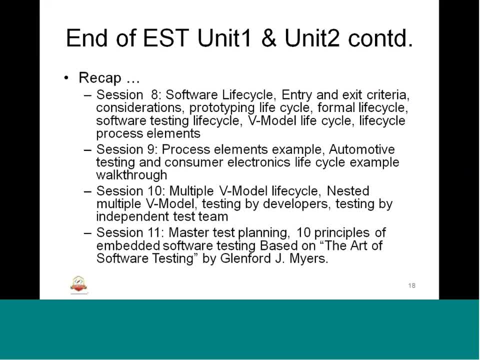 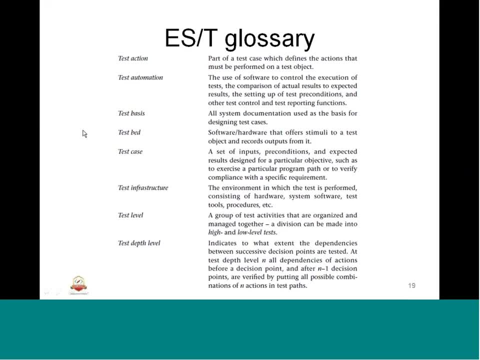 visited so far in the next session. so before concluding the class I will go through some of the classroom that we have for today. Test action: part of a test case which defines the actions that must be performed on a test. object: Test automation: we have seen use of software to control the execution of test, the comparison. 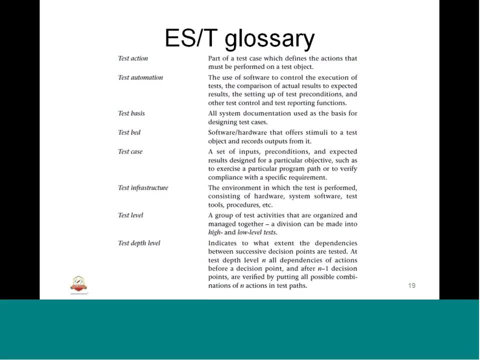 of actual test, actual results, the expected results, setting up of test speed conditions and other test control and test reporting functions. Test basis: all system recommendation used as the basis for designing test cases. Testbed software hardware is a both that offers stimuli to a test object and records the output. 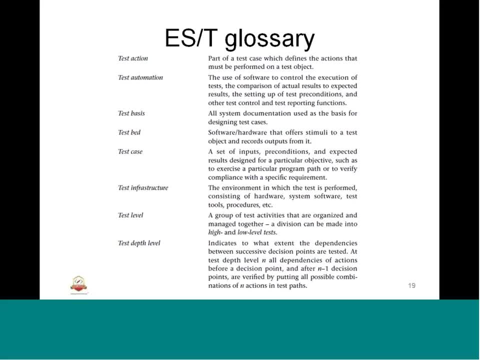 on that Test case, we know that it is set of inputs, preconditions and expected results designed for a particular objective or a requirement, such as to exercise a particular program path or to verify compliance with a specific requirement. We know that requirement level. we have a high level test or a block box system. we will 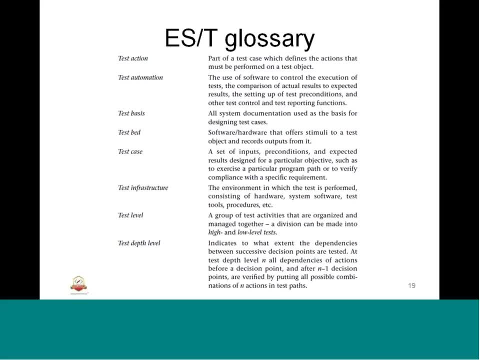 have a test case. We will do the test cases accordingly and provide block testing. we will do the coverage and all that while doing the execution on the implementation of the code. Test infrastructure- the environment in which the test is performed consisting of hardware. 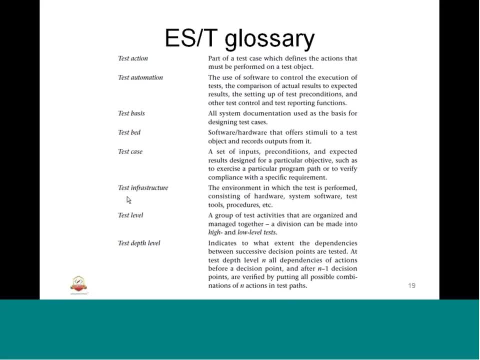 system, software test tools, test tools procedures, etcetera. with the help of infrastructure, we develop or build the environment. it also has a automation aspects involved. Hey, well, we have seen for earlier sessions a group of test activities that are organized. 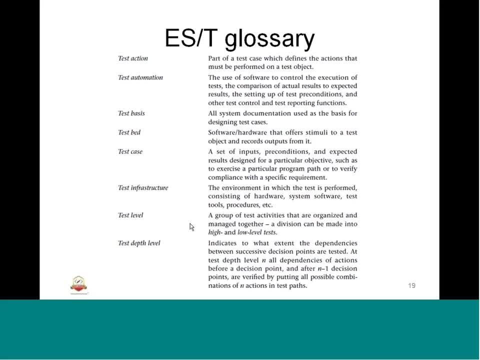 and managed together, division can be made into high level. Then we have a test depth level indicates to what extent it dependencies between perfect decision point of s At test depth level n, all dependencies of actions before descending point and after n-1 position point. 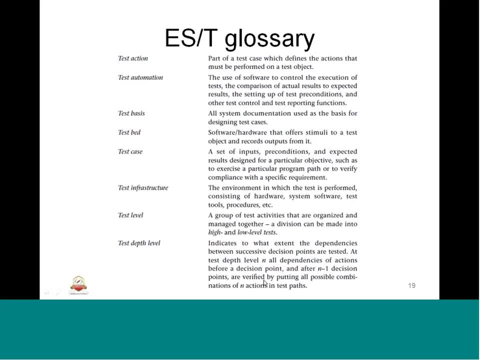 Now we are getting expressed by putting all possible combinations on the test point, combinations of N actions in that test path. so that is about the glossary that we have discussed today. So with this we come to the end of this today's session and the units that we have completed. 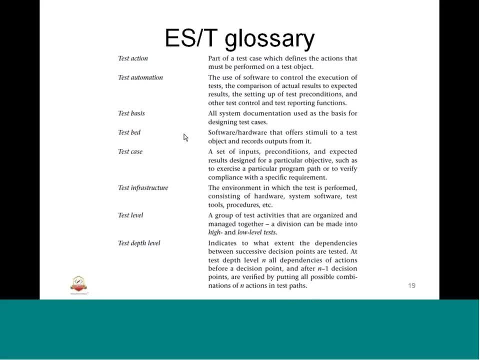 unit 1 and unit 2, we will do a small recap of whatever the units and sessions we have completed and we will take up the next unit, that is, static analysis, inspection and reviews, in the next session.